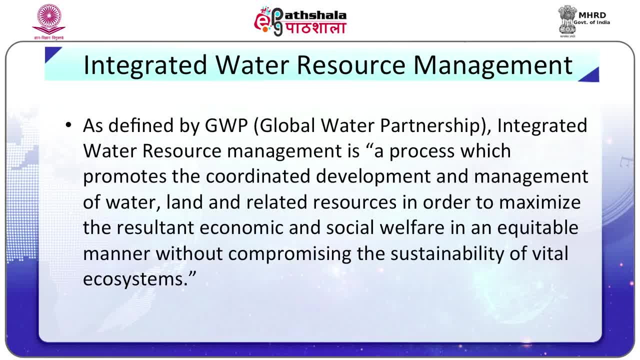 As defined by GWP, which is Global Water Partnership. integrated water resource management is a process which promotes the coordinated development and management of water, land and related resources in order to maximize the resultant economic and social welfare in an equitable manner, without compromising the sustainability of vital ecosystems. 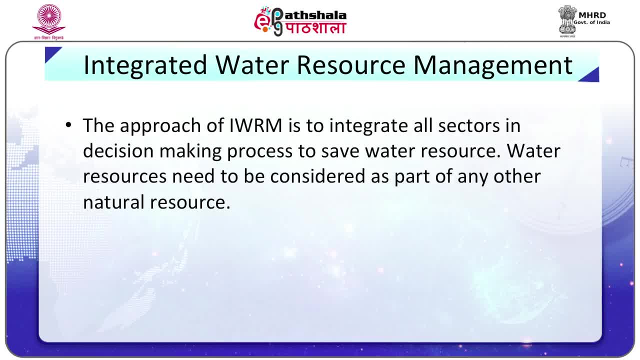 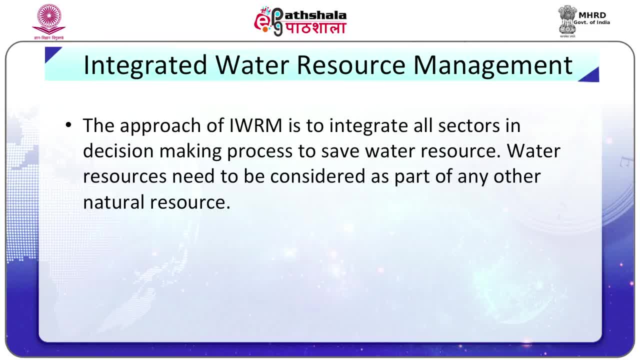 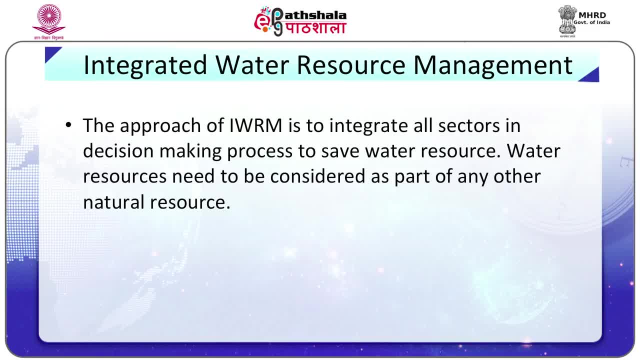 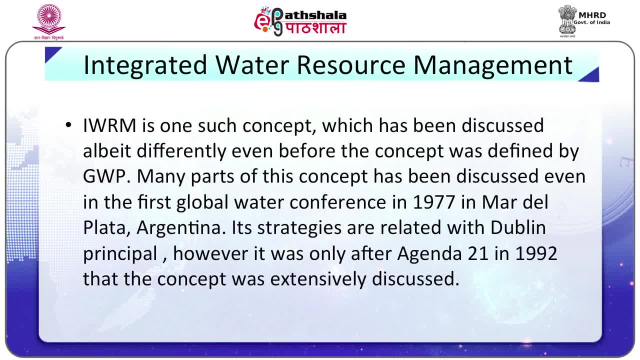 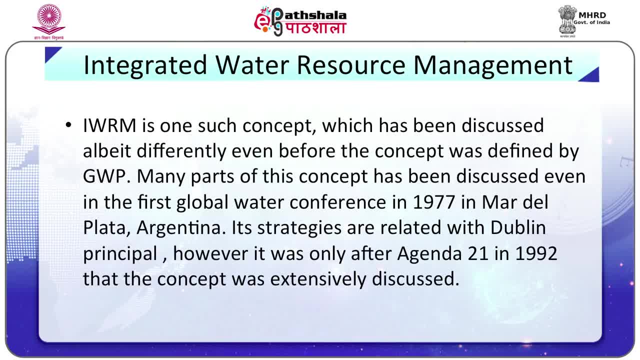 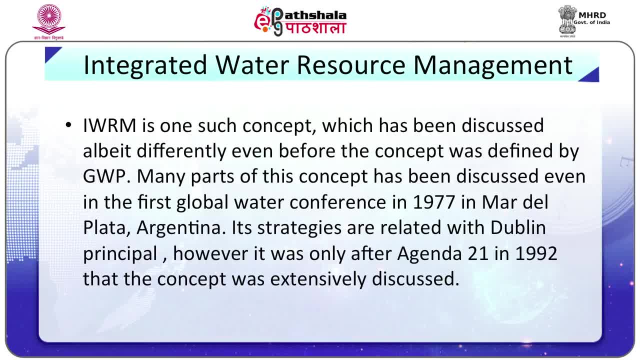 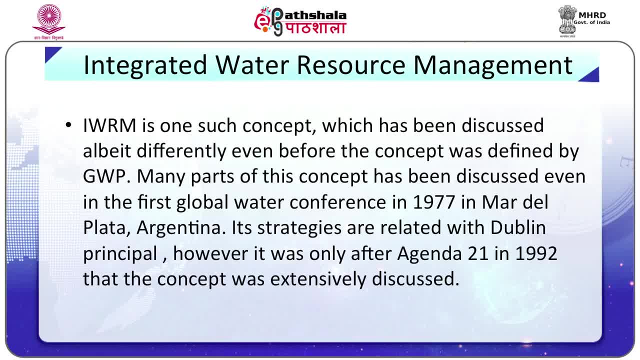 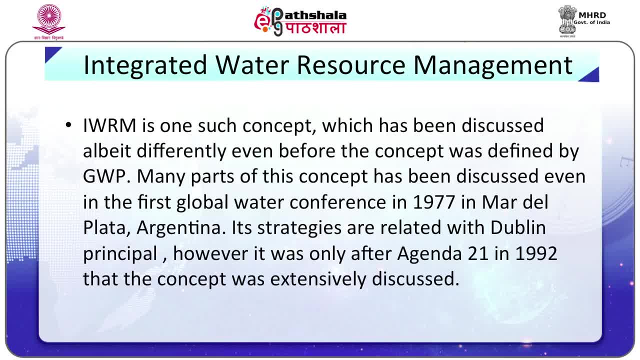 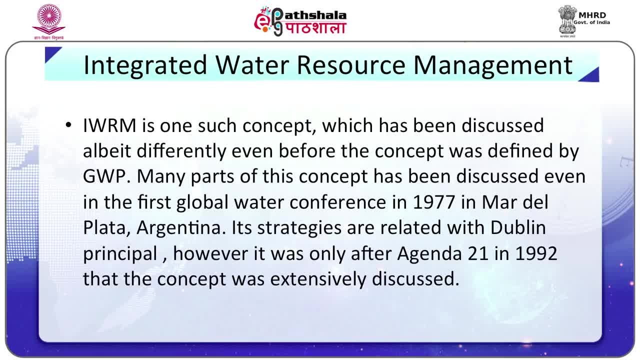 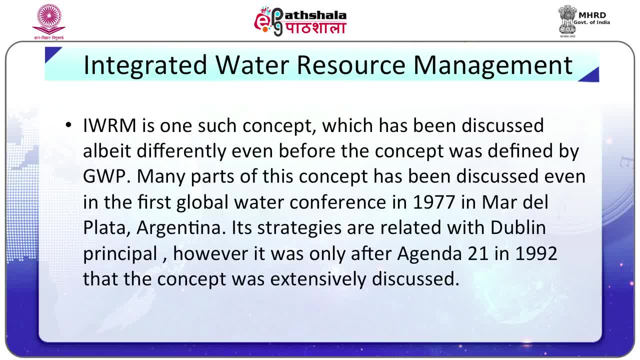 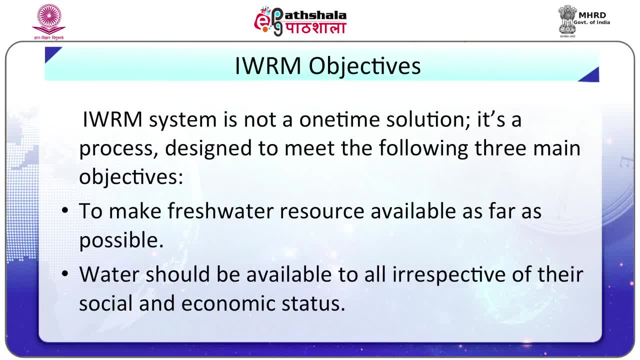 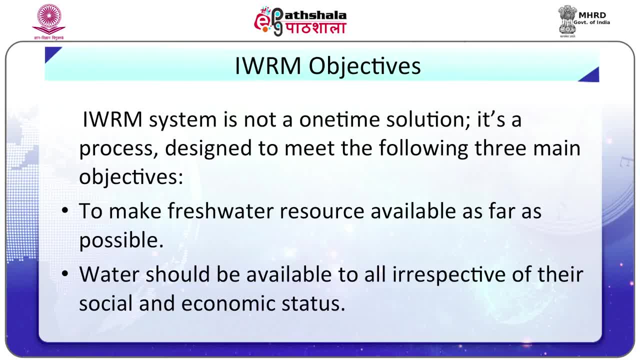 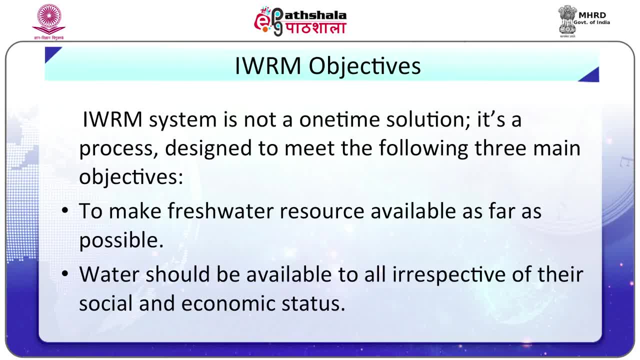 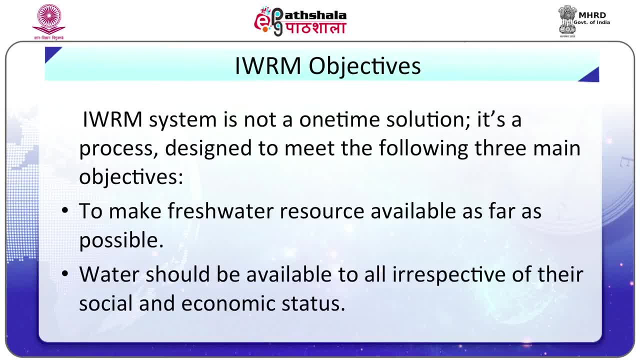 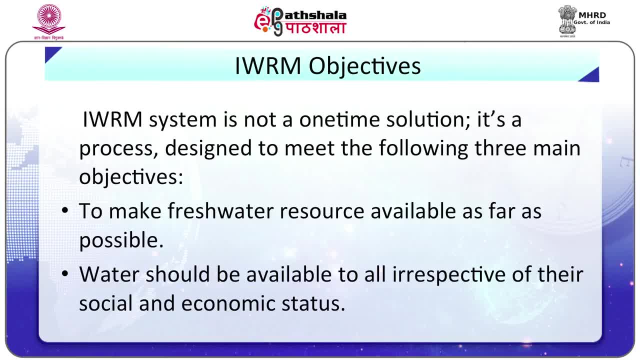 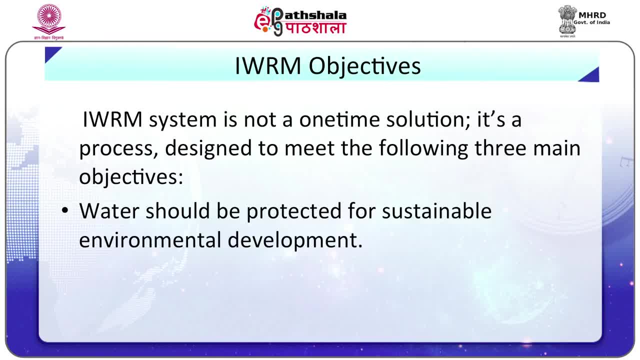 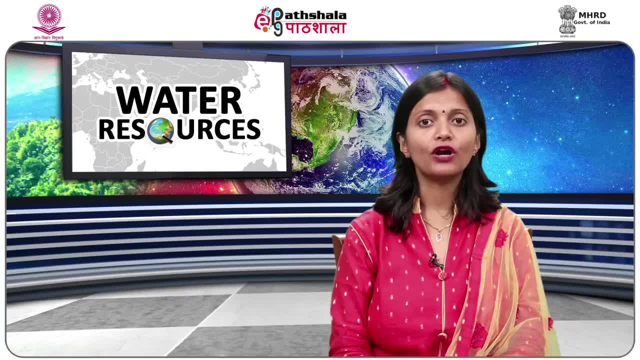 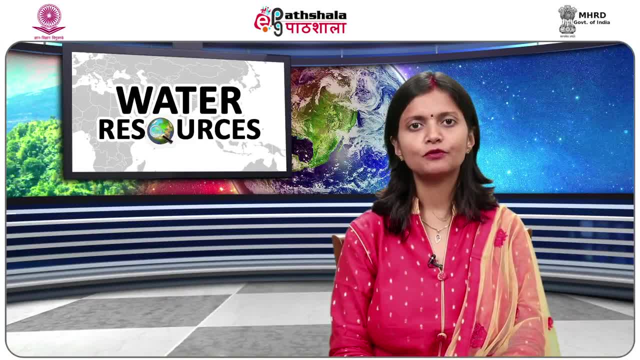 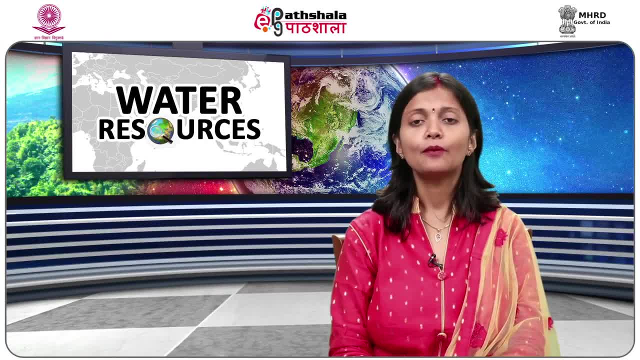 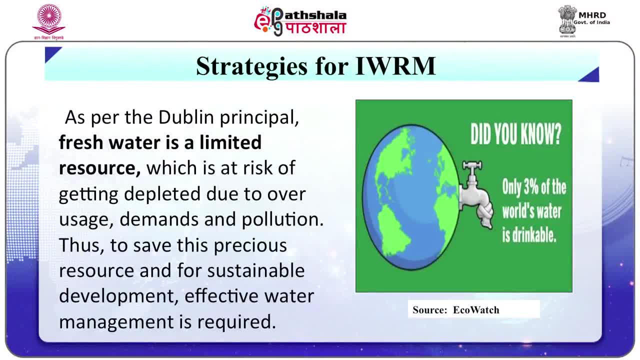 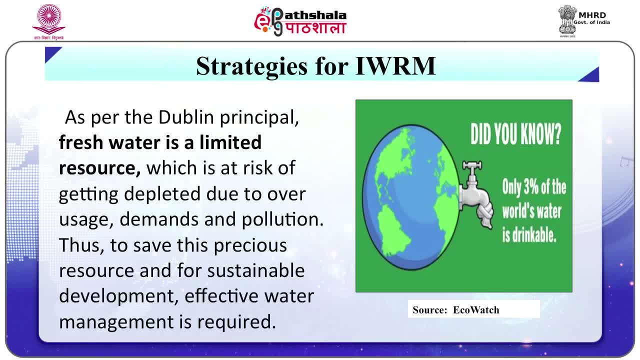 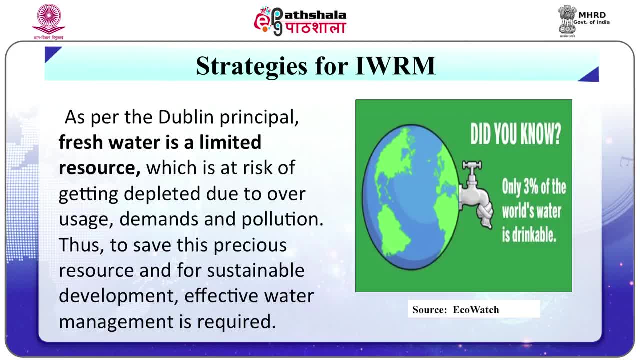 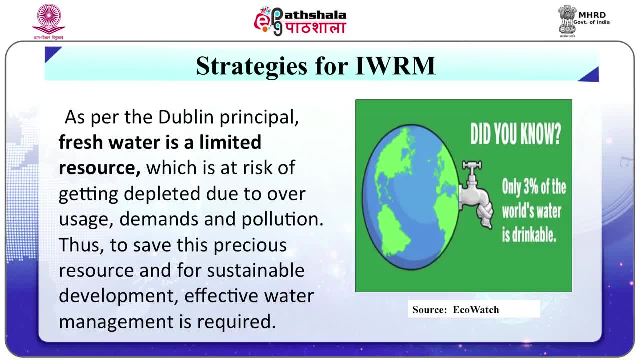 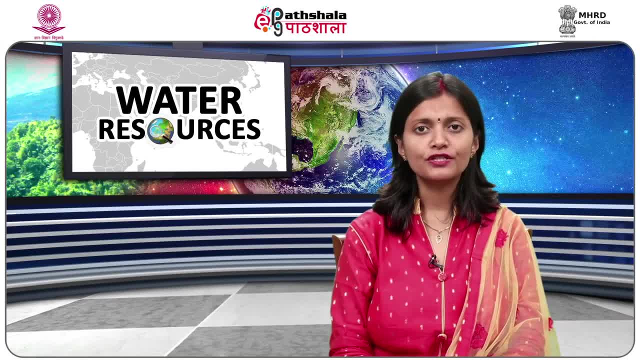 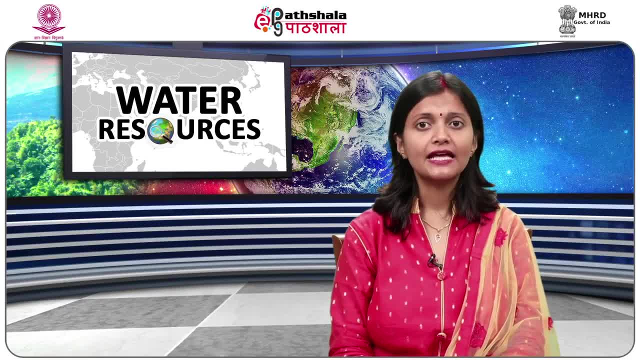 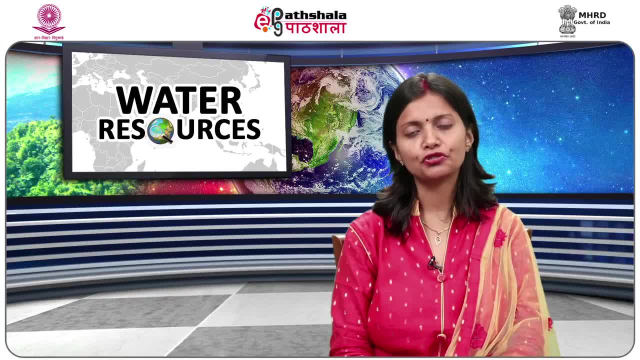 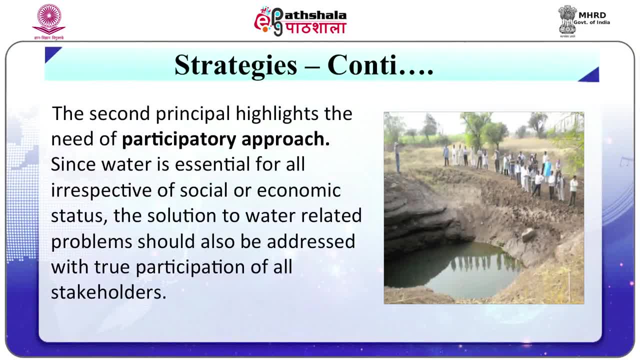 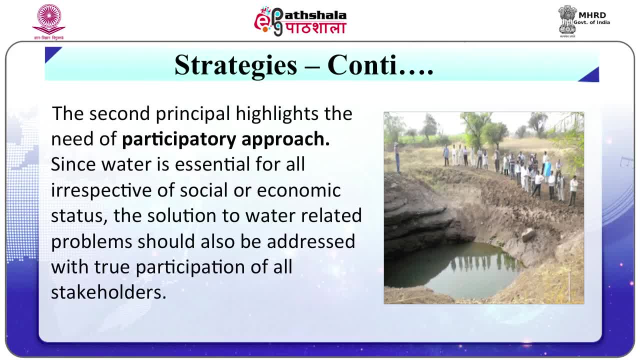 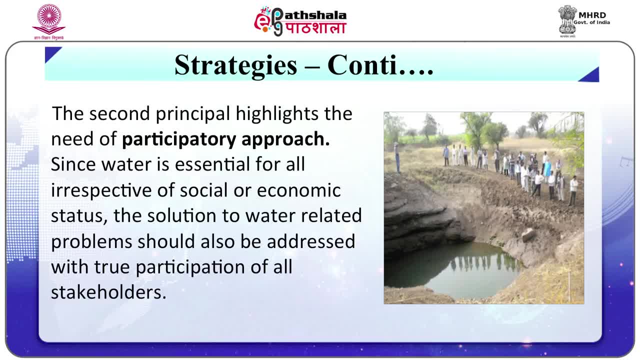 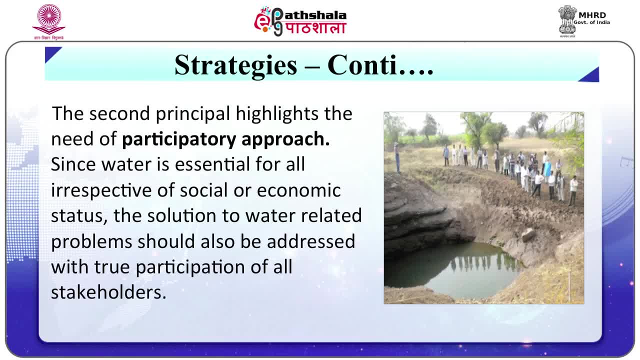 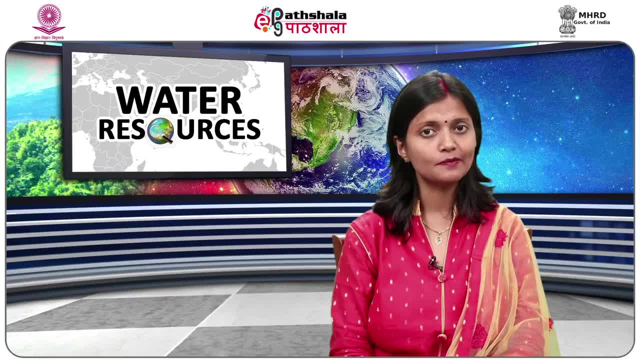 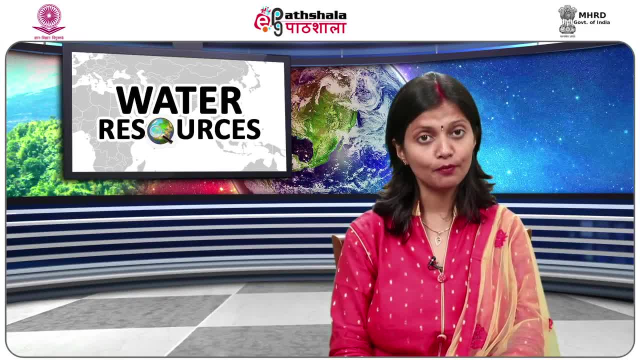 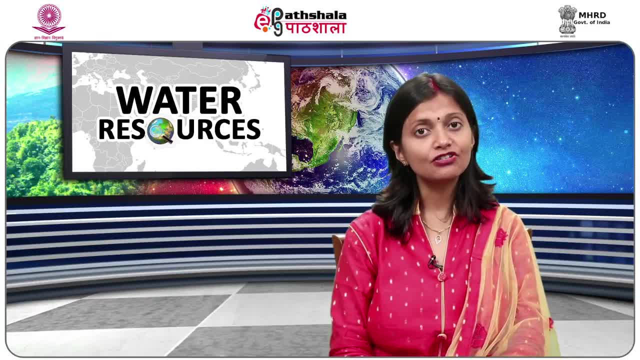 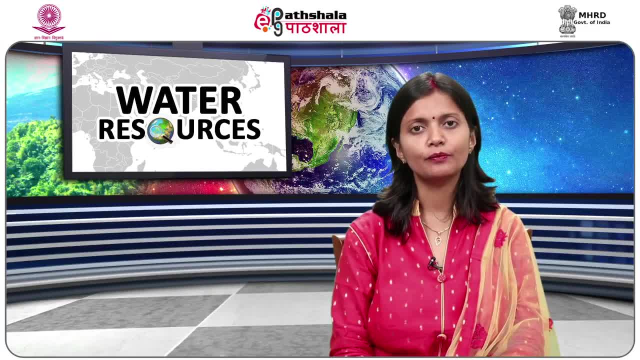 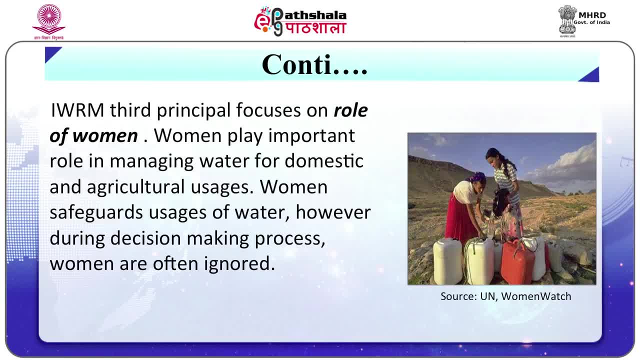 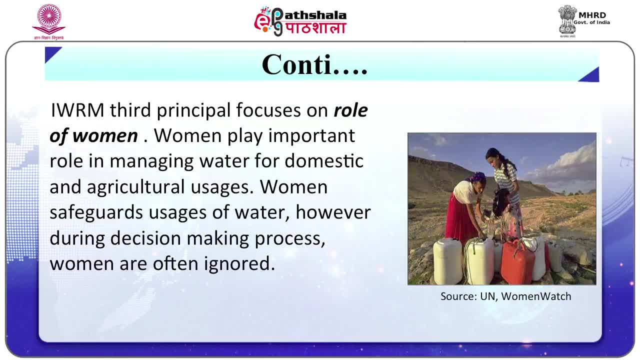 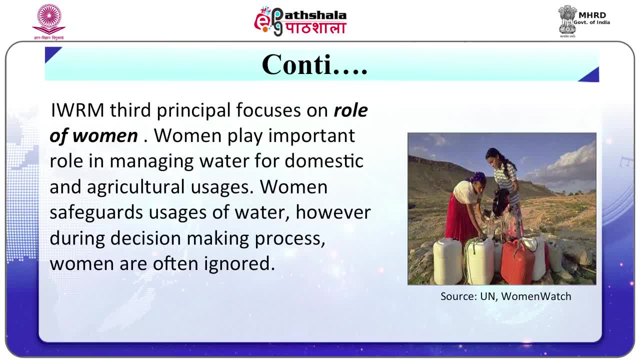 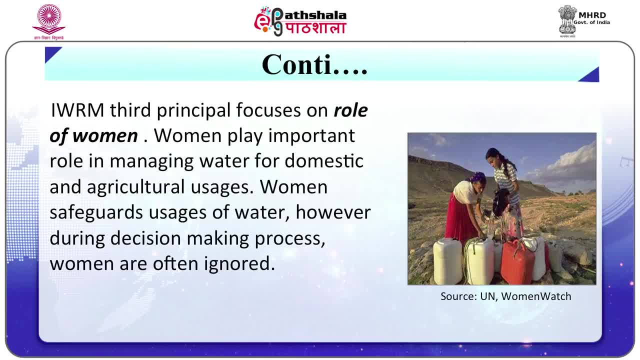 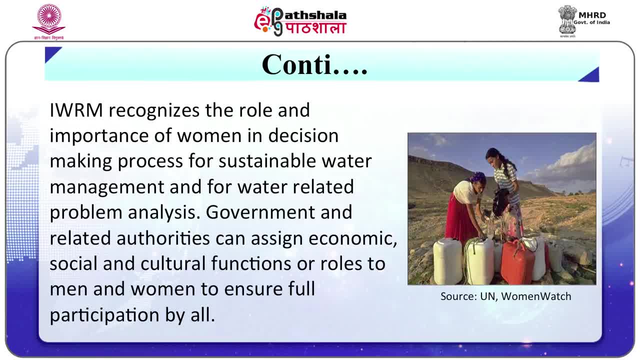 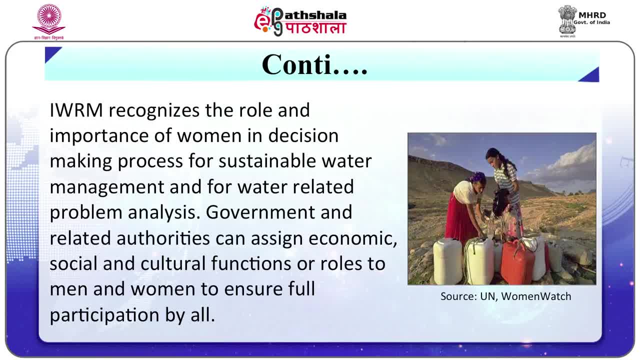 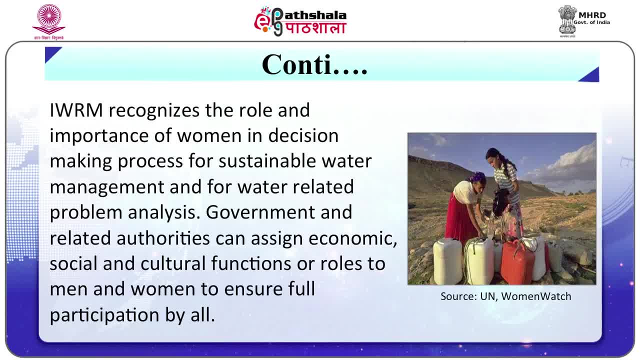 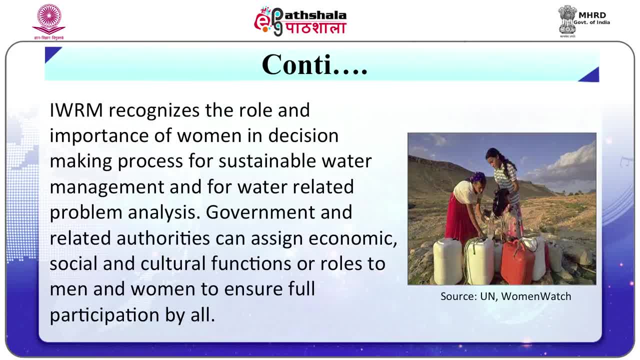 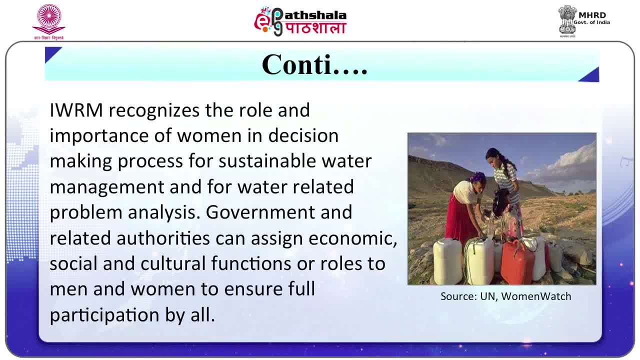 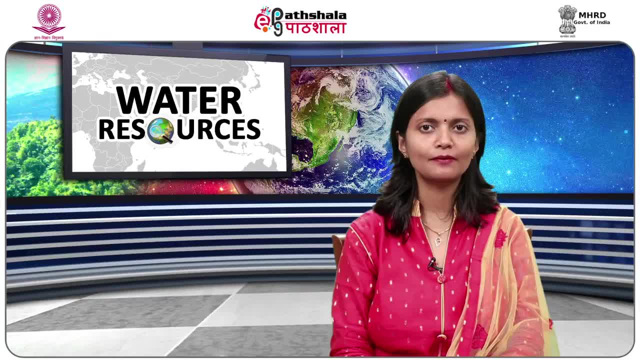 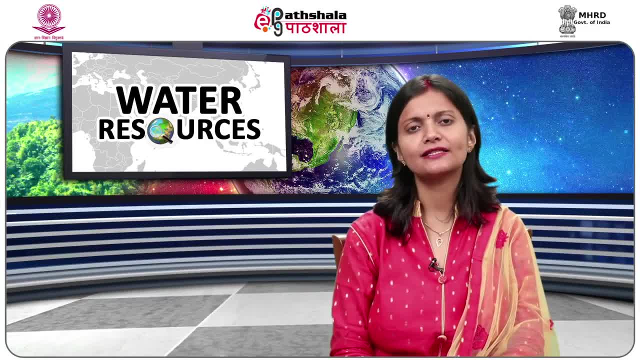 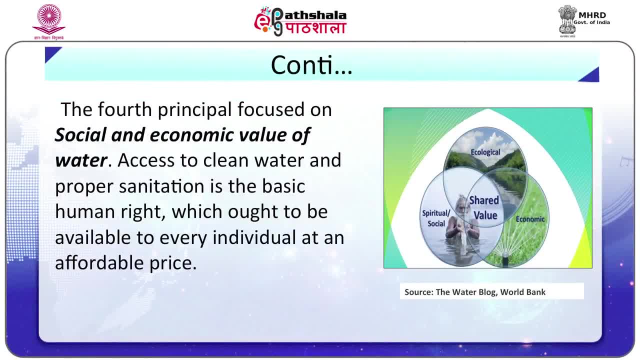 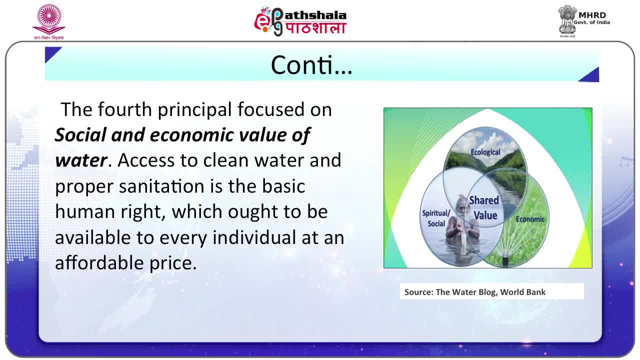 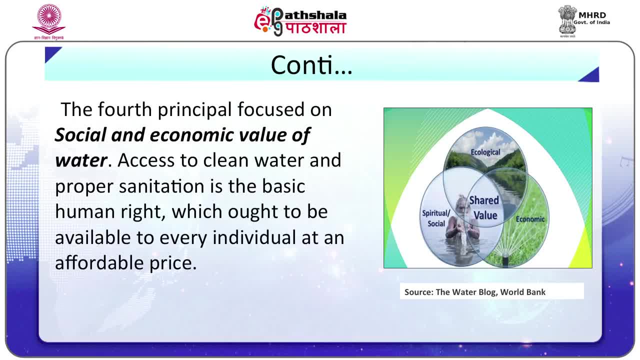 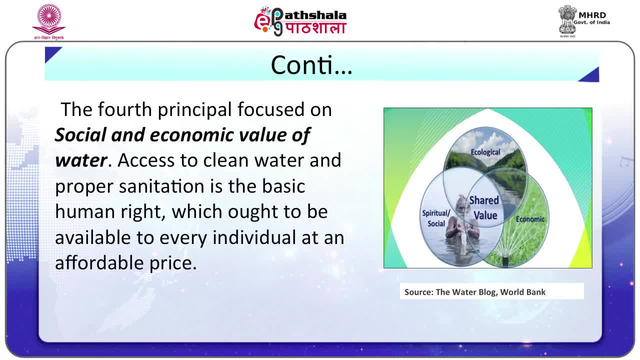 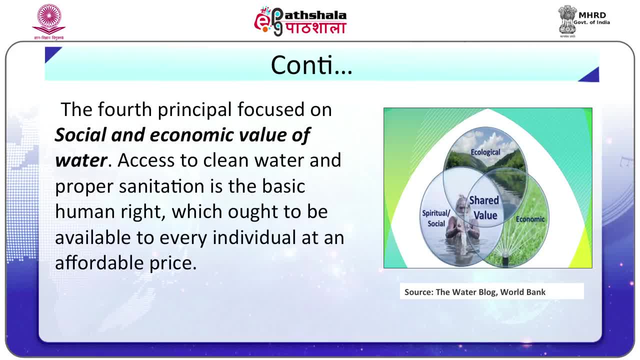 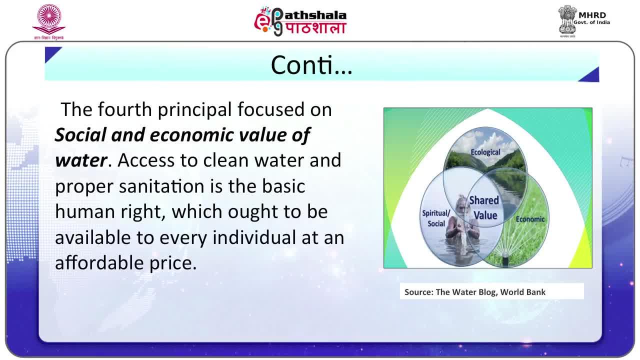 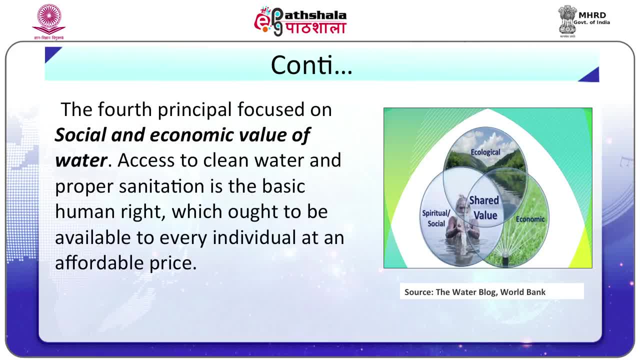 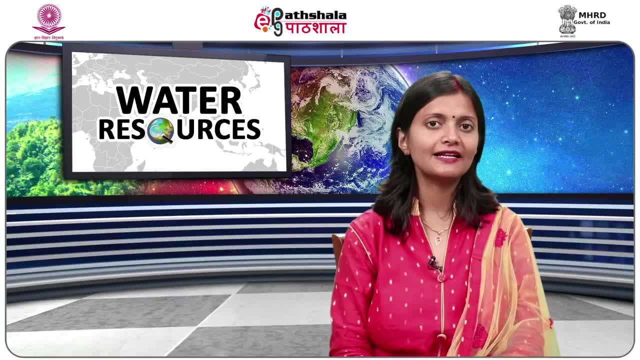 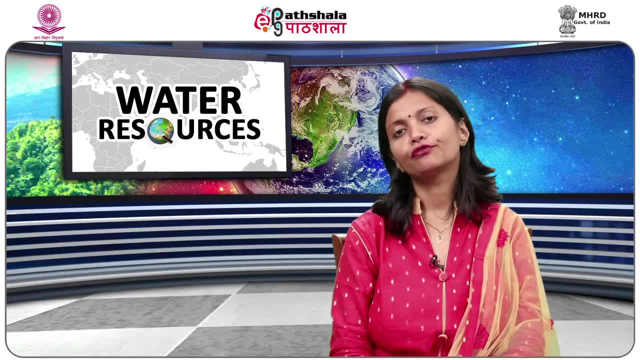 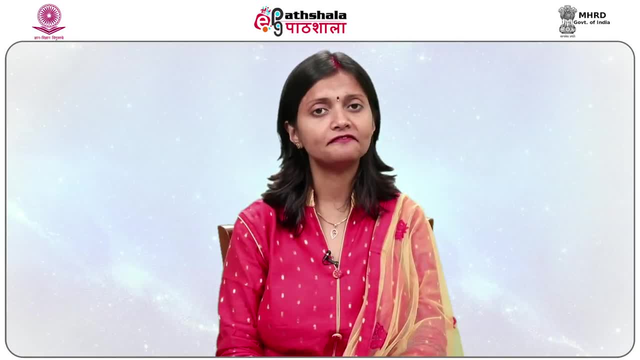 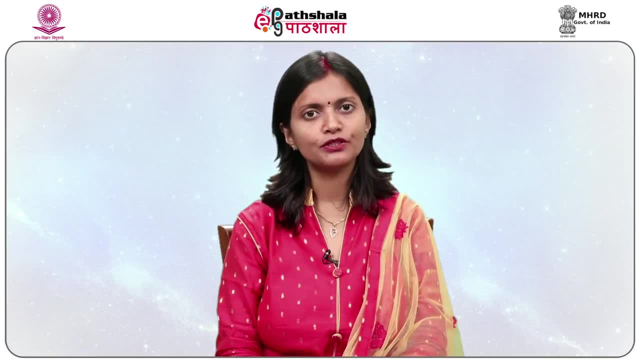 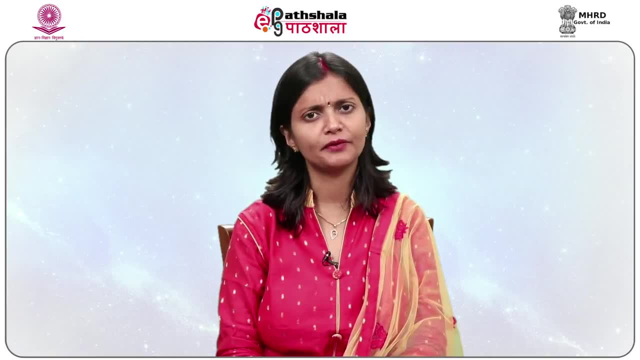 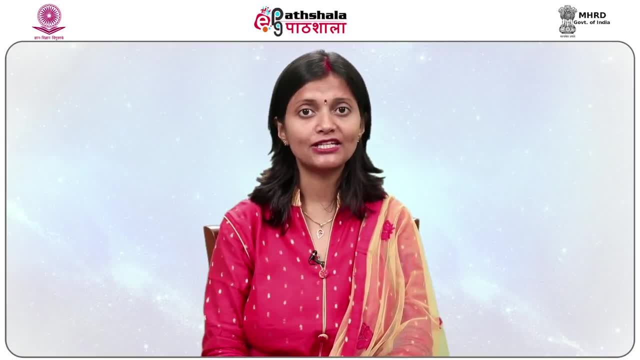 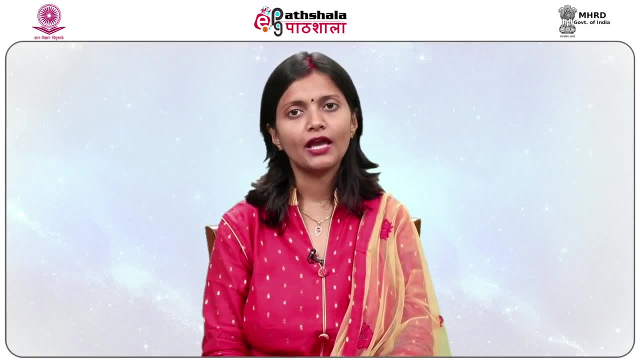 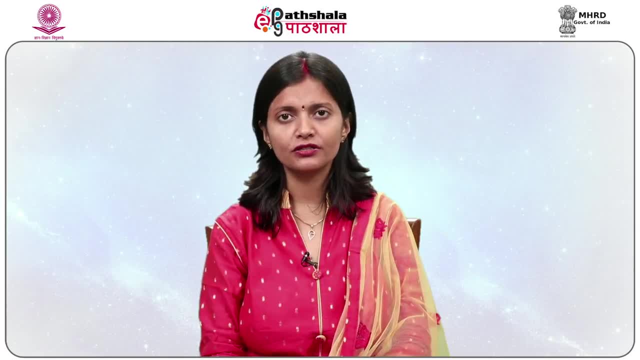 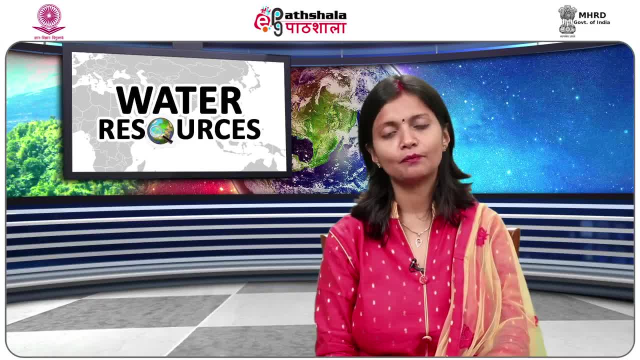 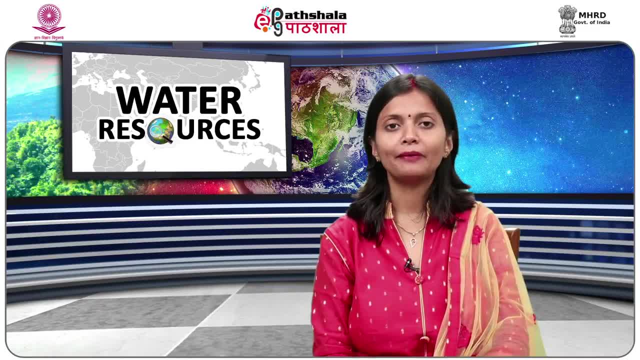 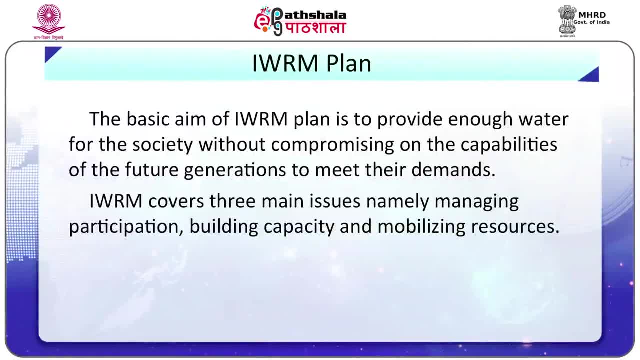 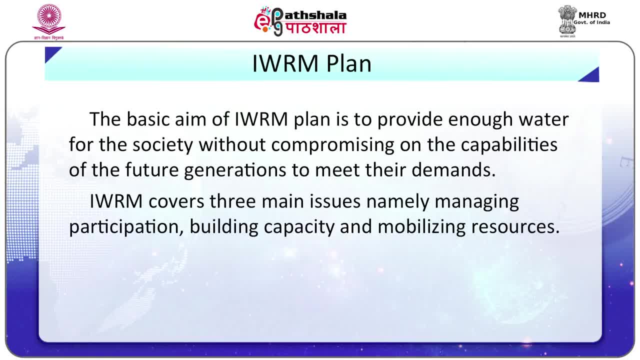 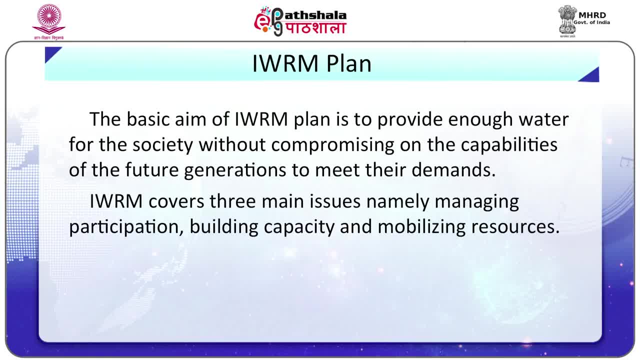 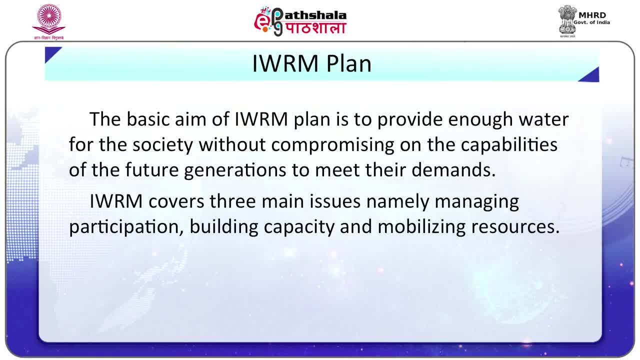 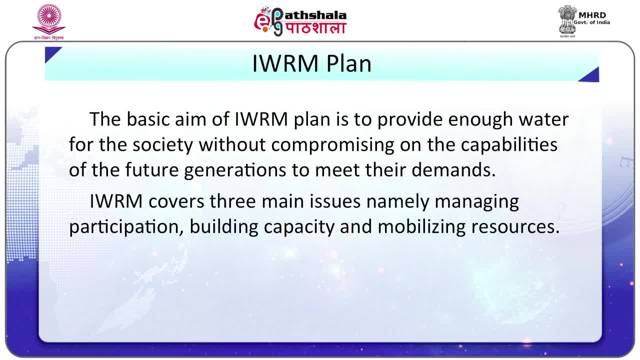 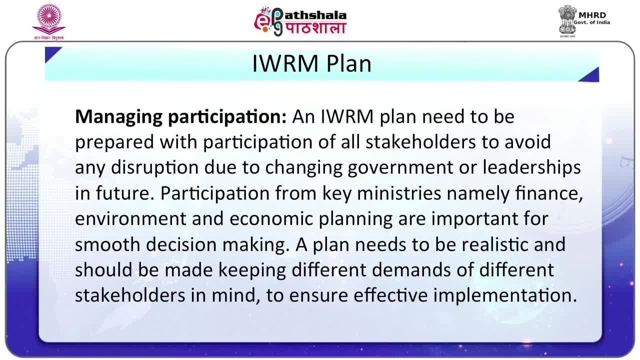 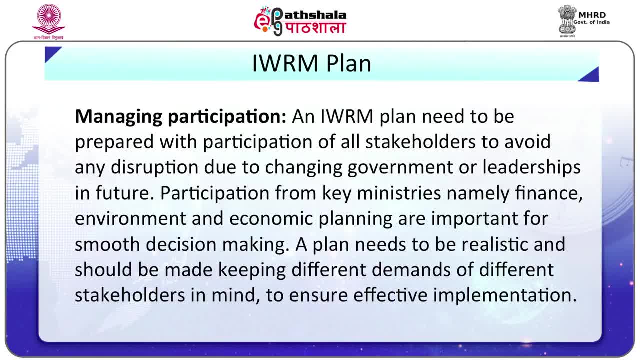 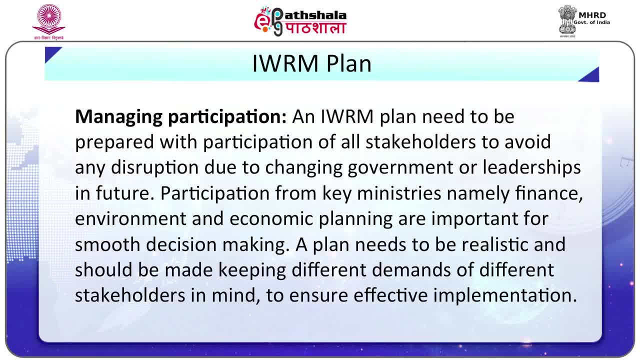 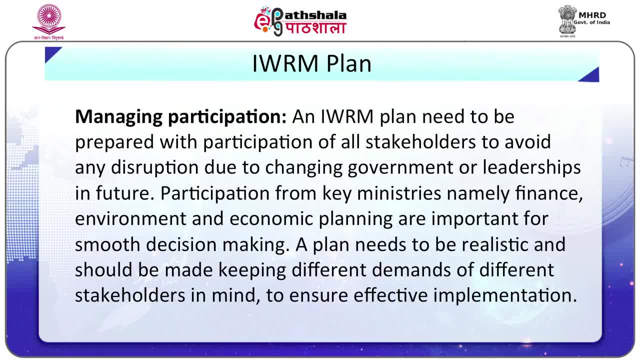 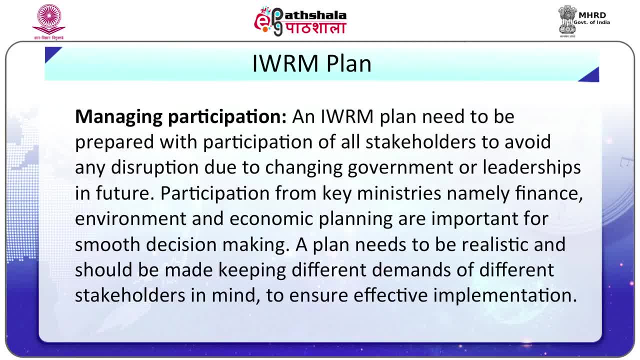 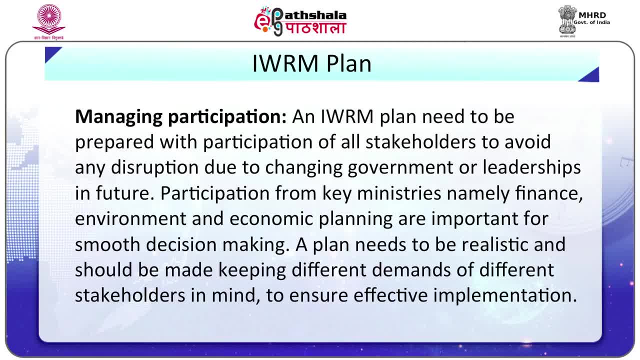 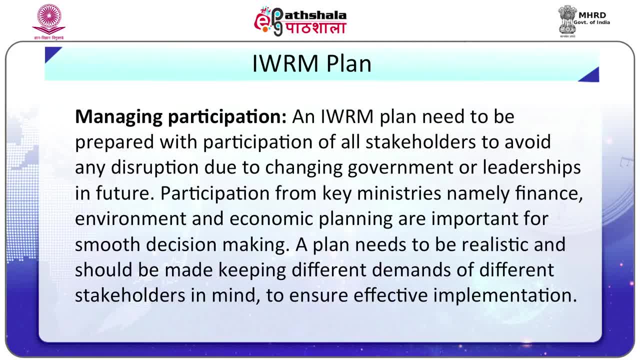 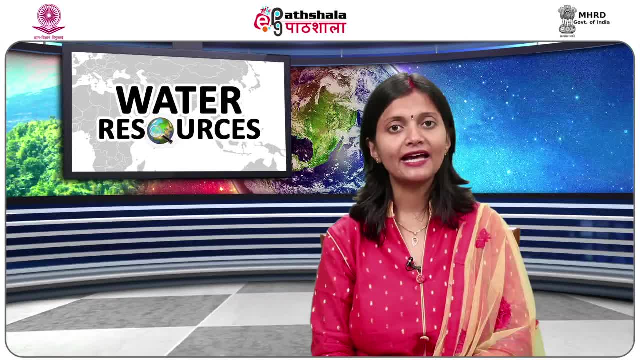 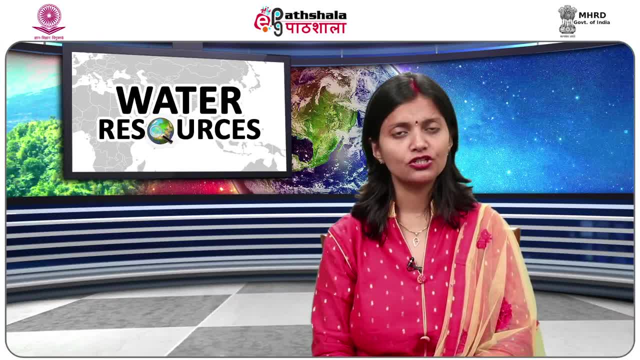 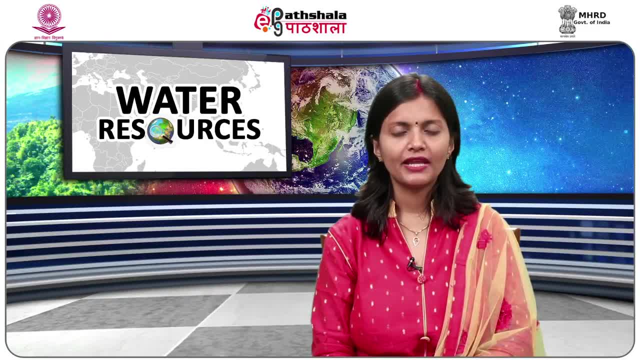 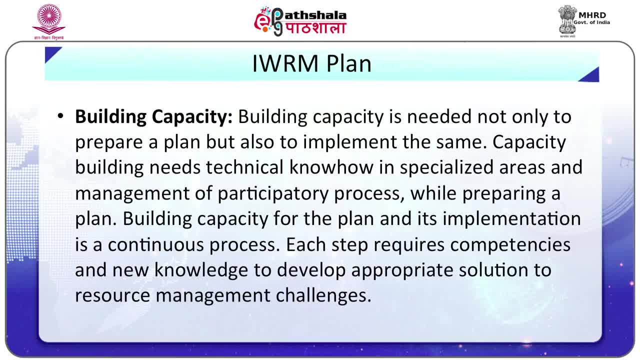 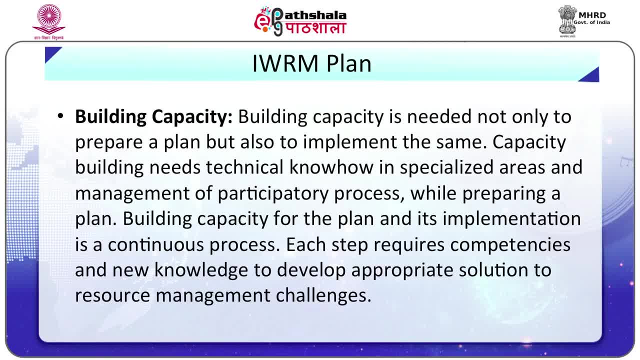 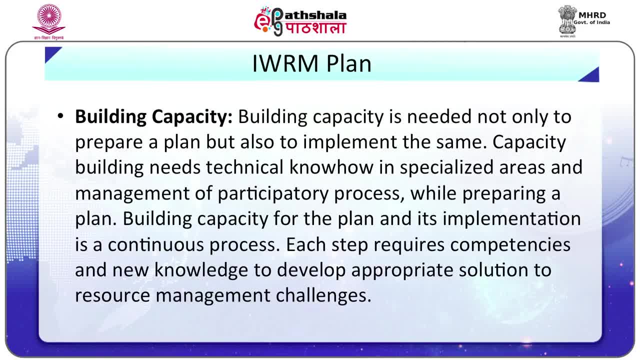 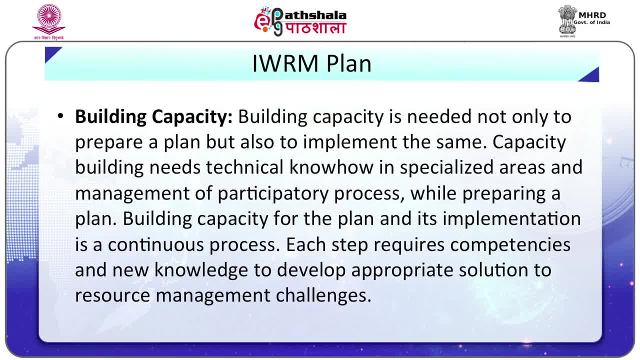 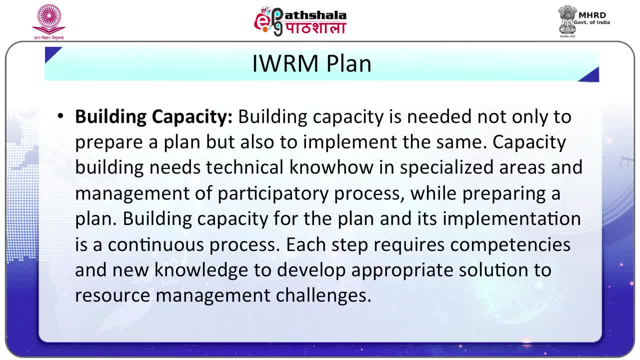 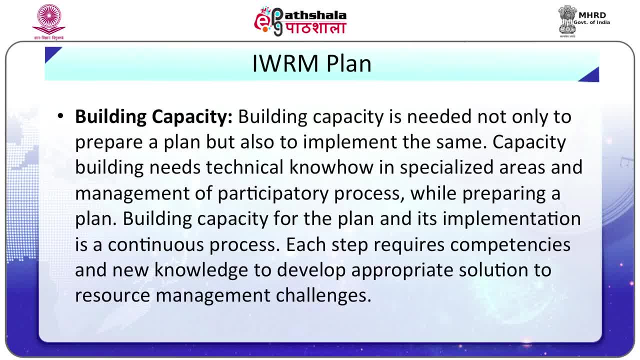 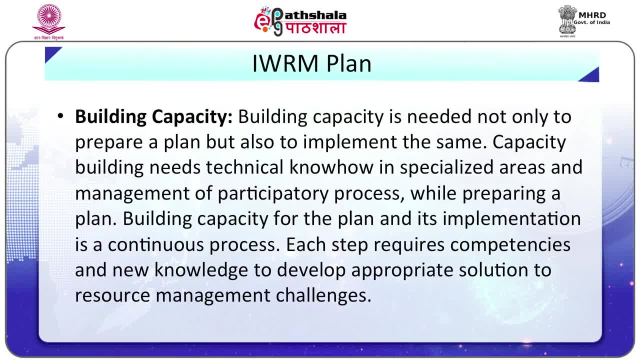 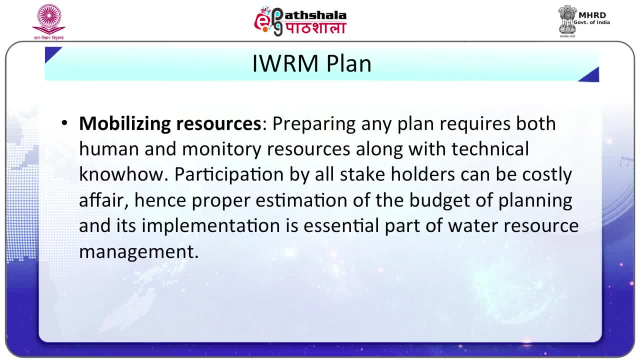 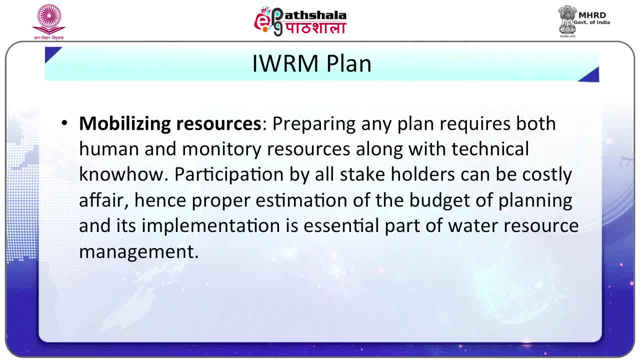 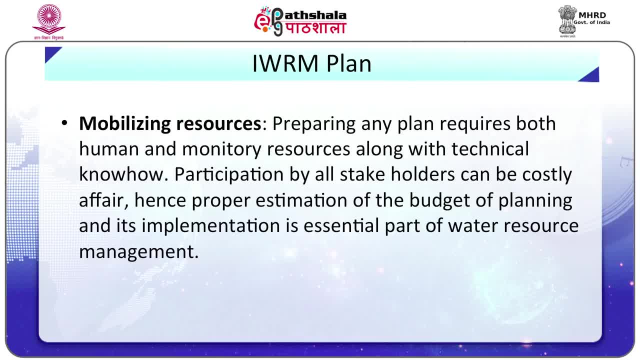 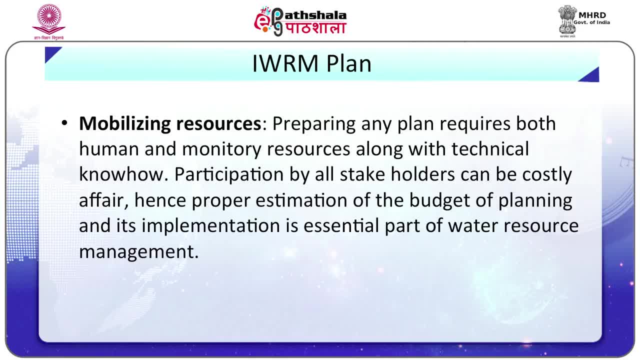 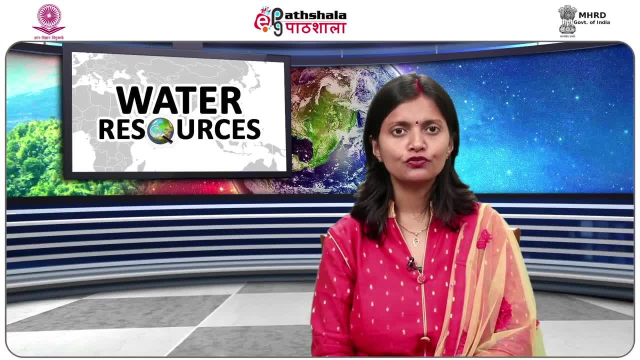 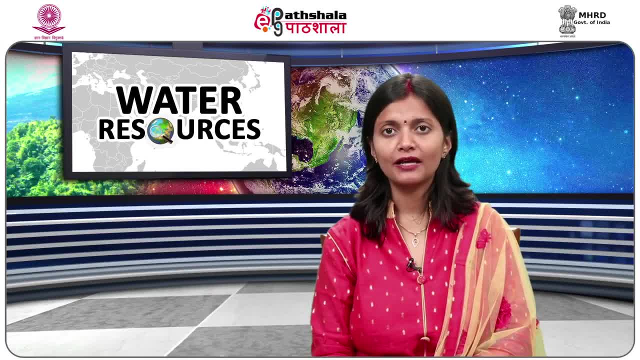 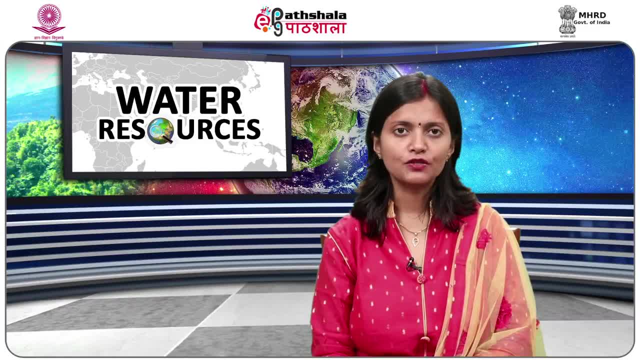 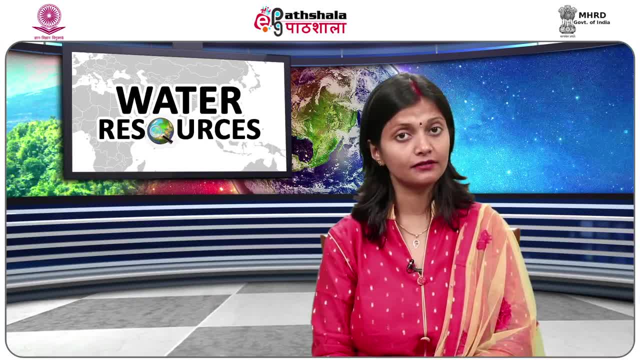 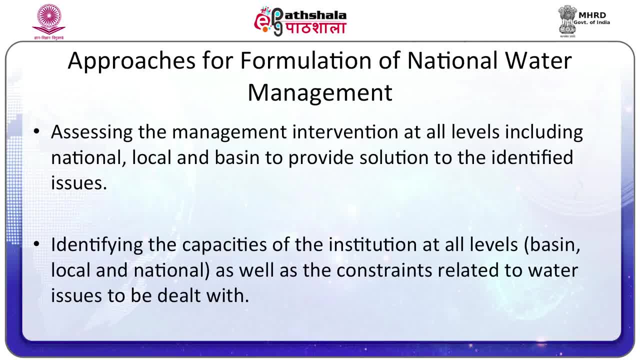 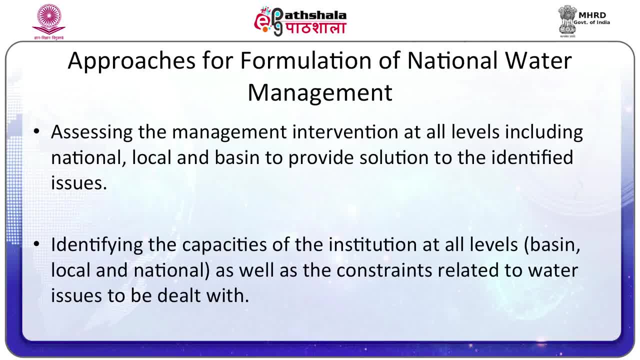 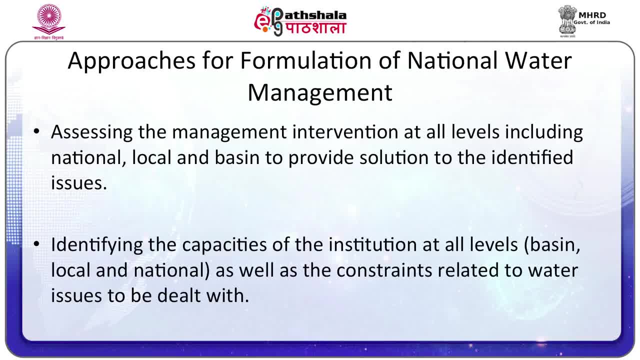 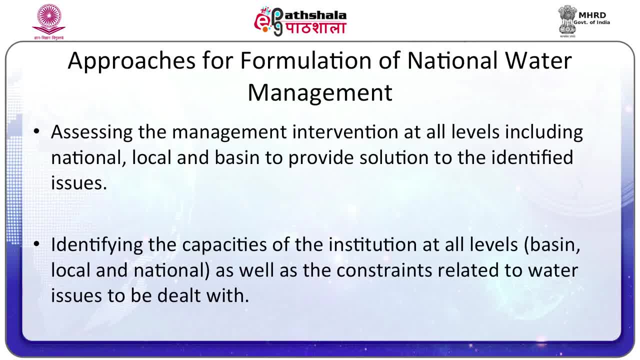 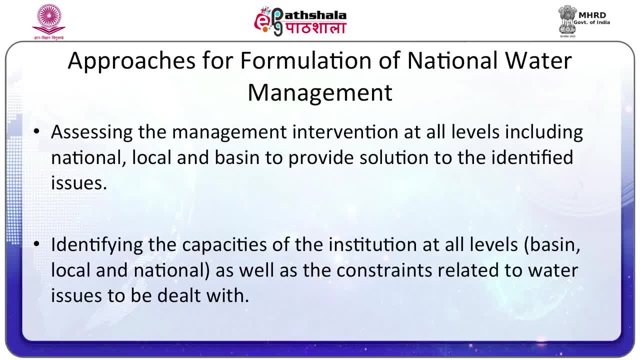 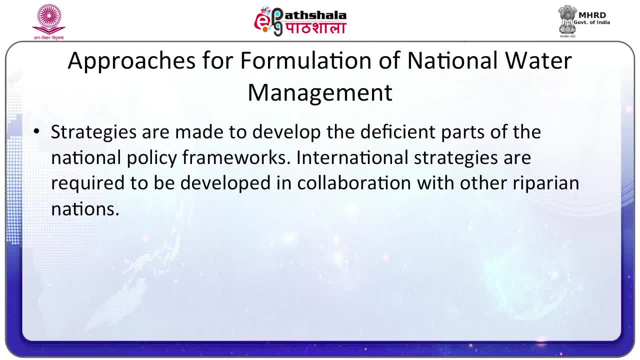 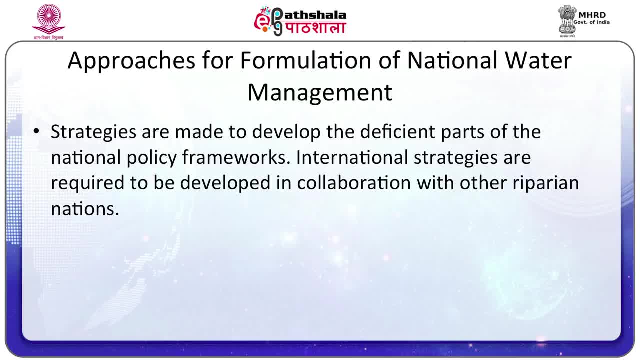 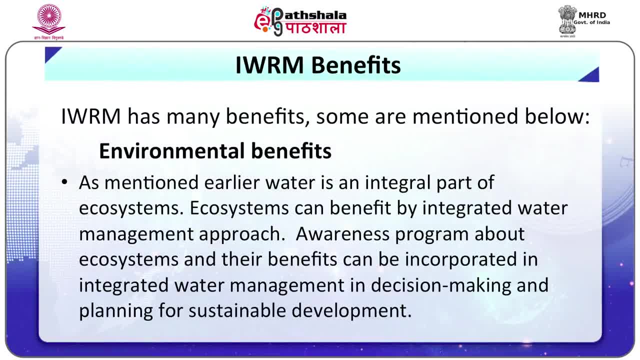 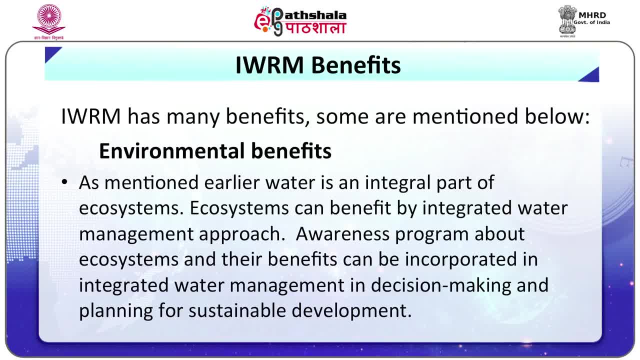 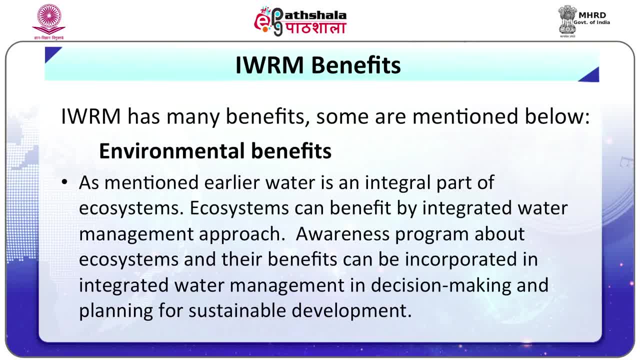 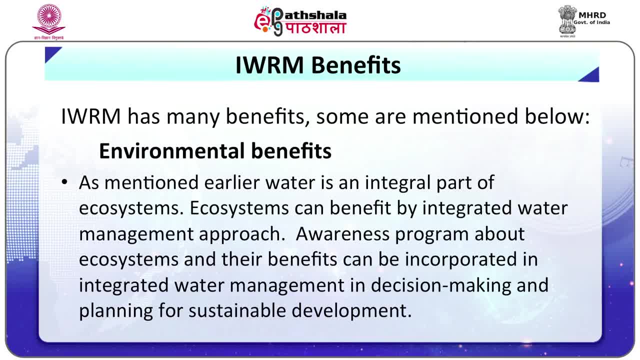 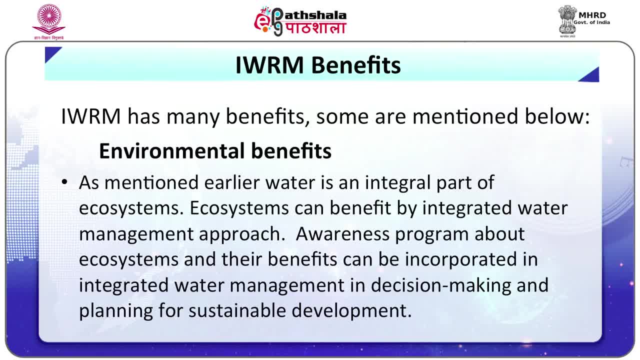 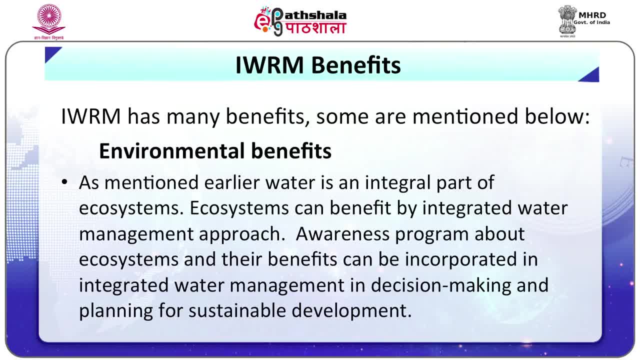 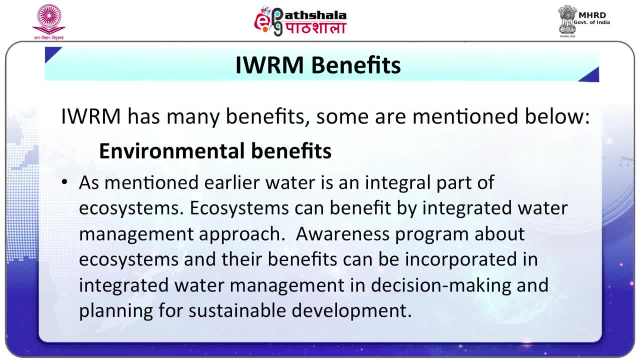 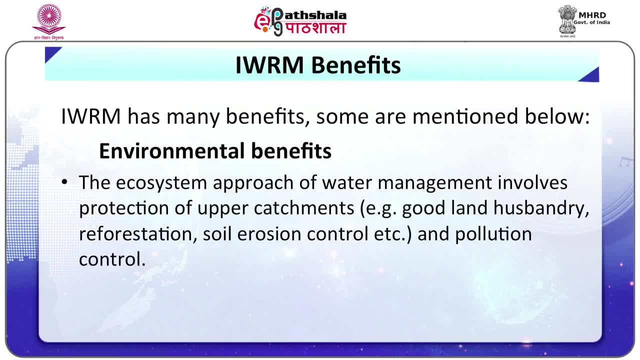 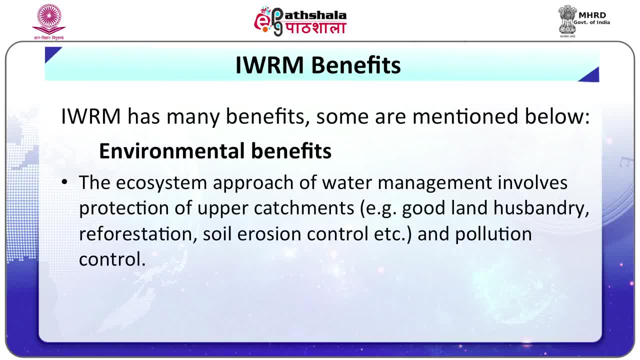 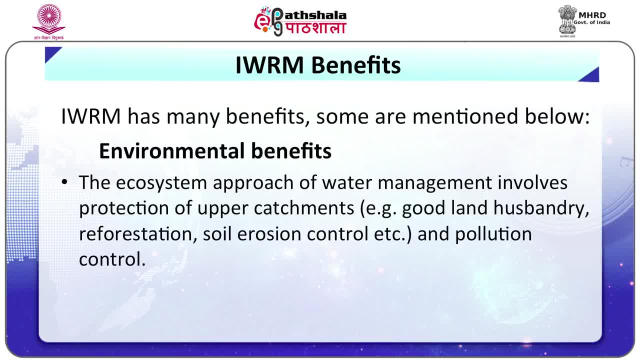 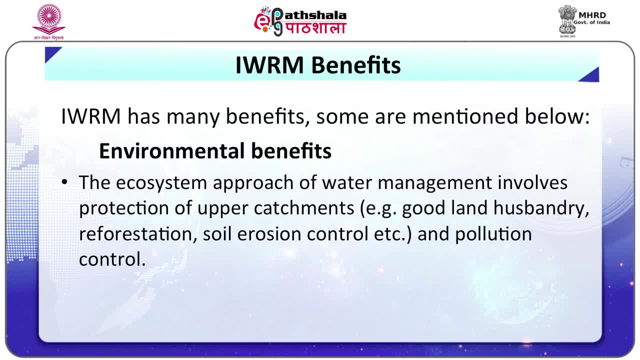 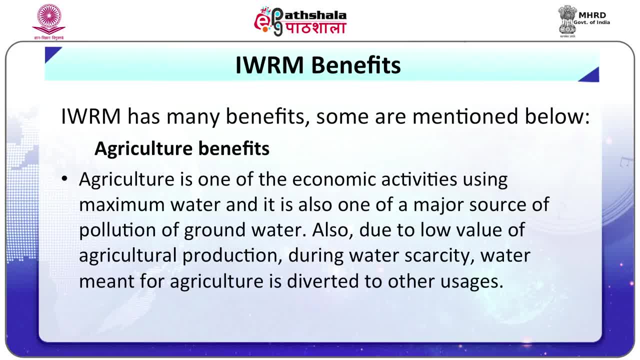 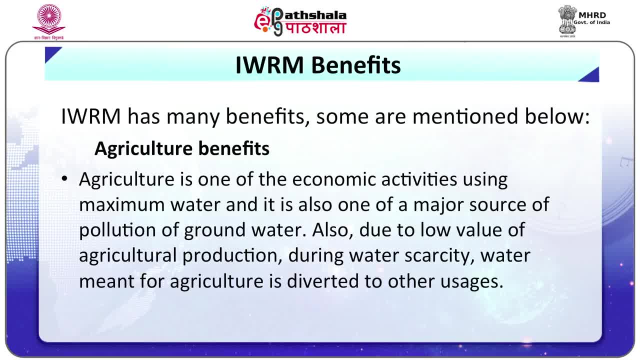 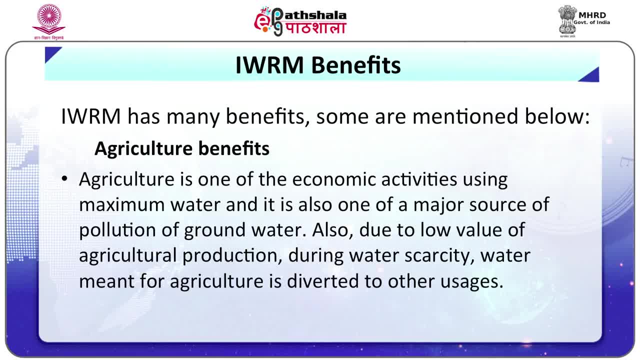 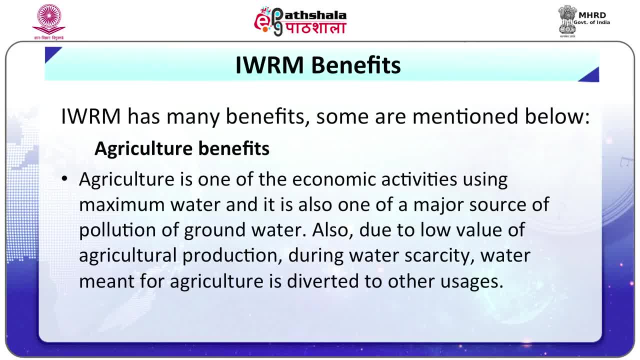 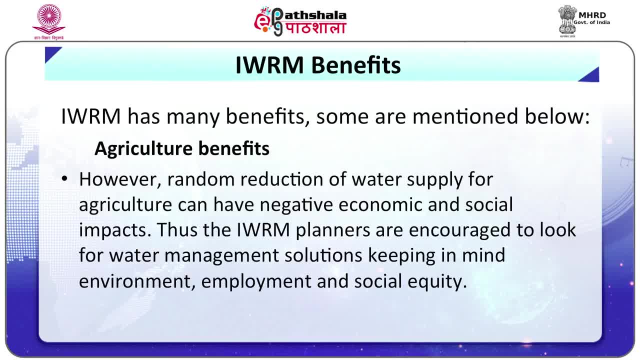 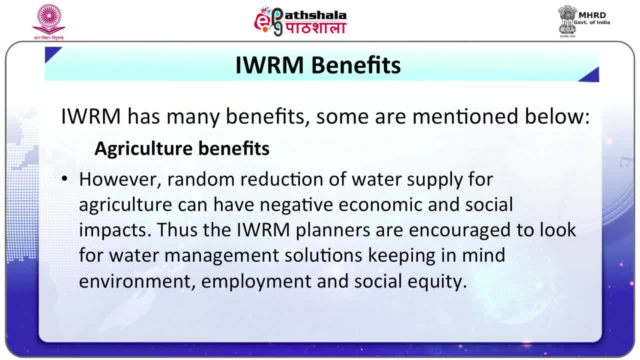 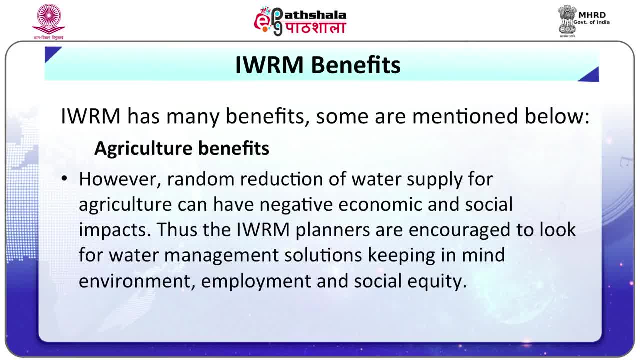 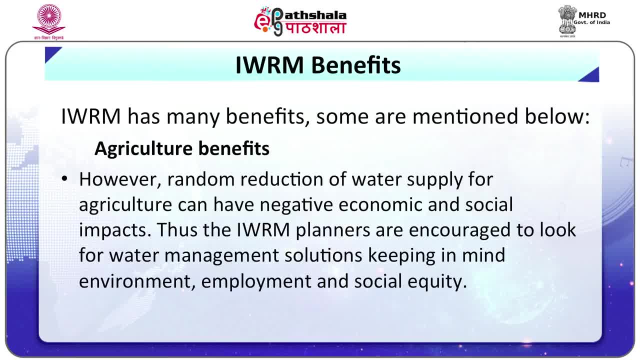 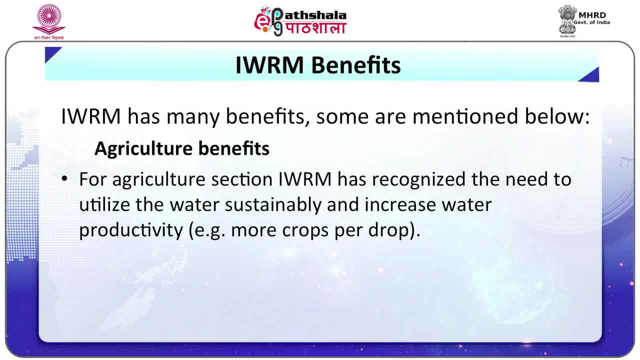 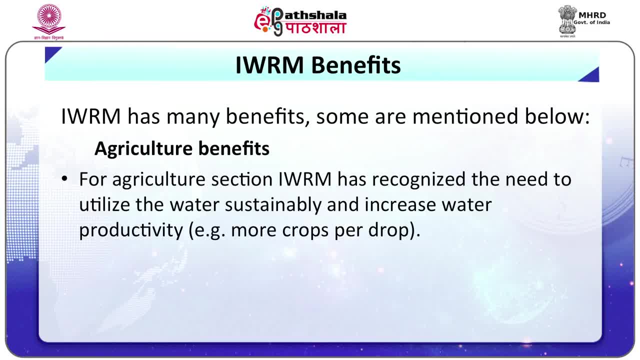 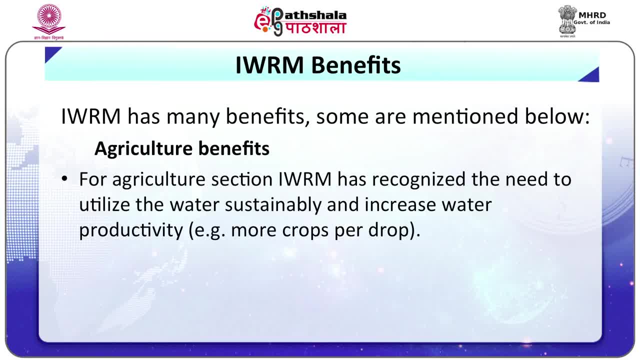 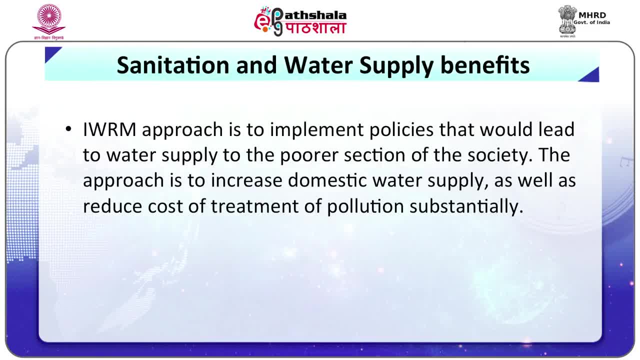 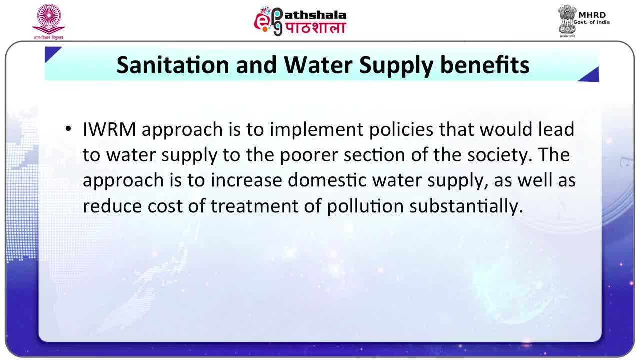 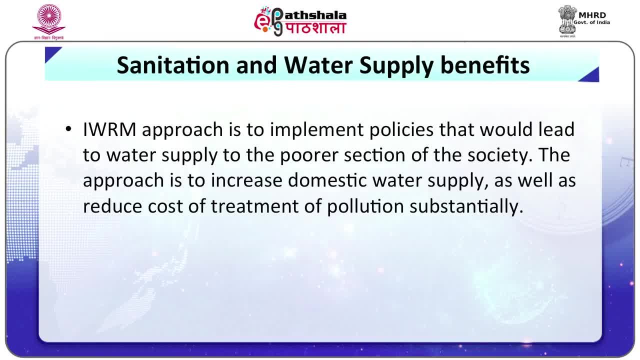 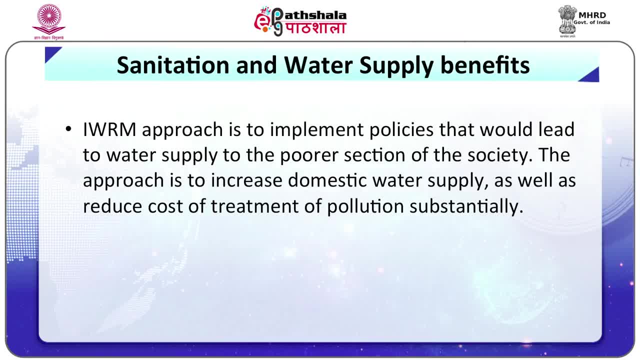 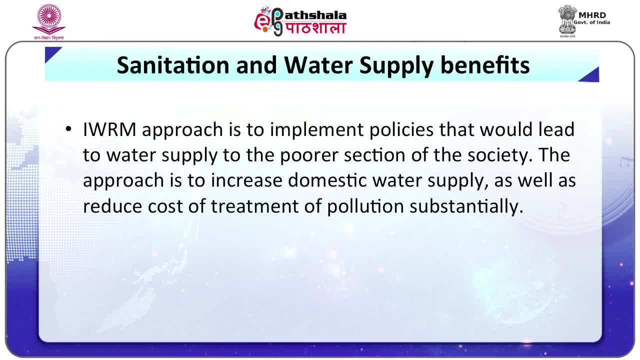 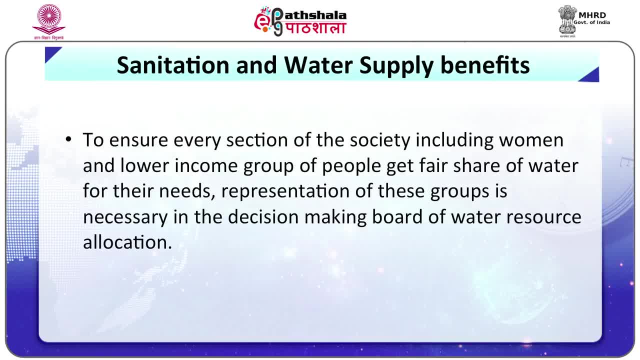 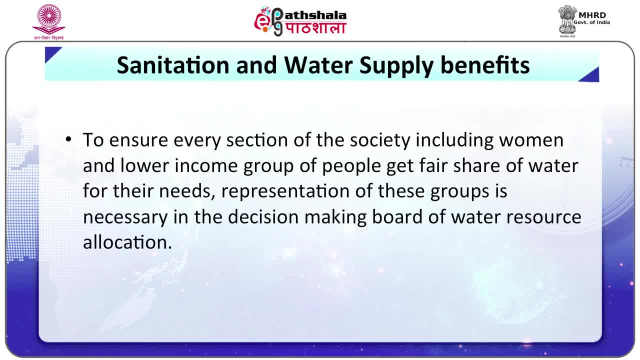 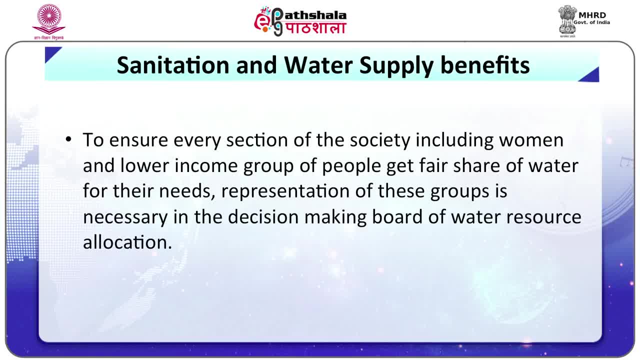 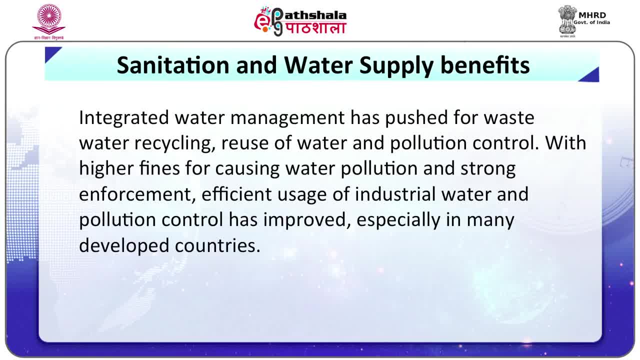 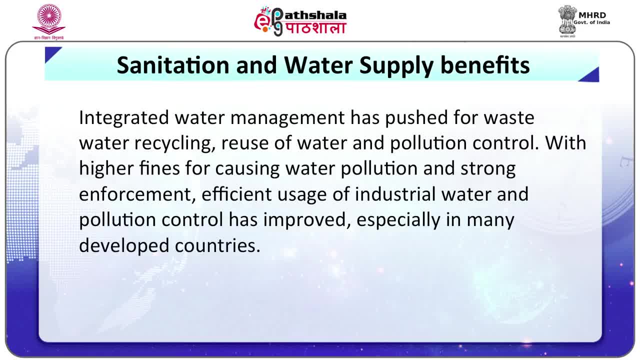 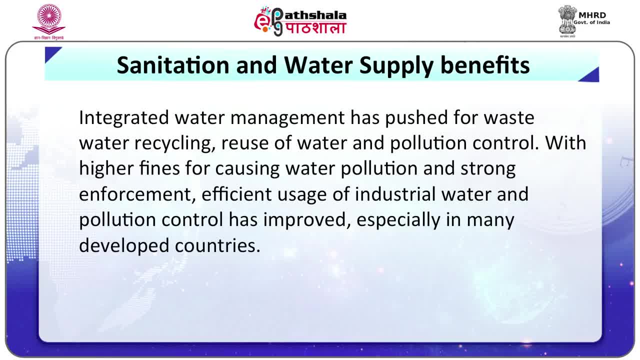 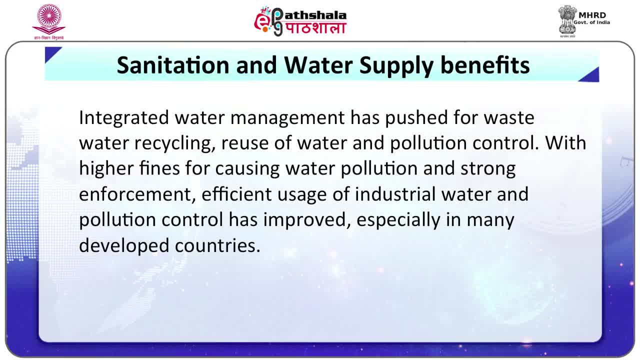 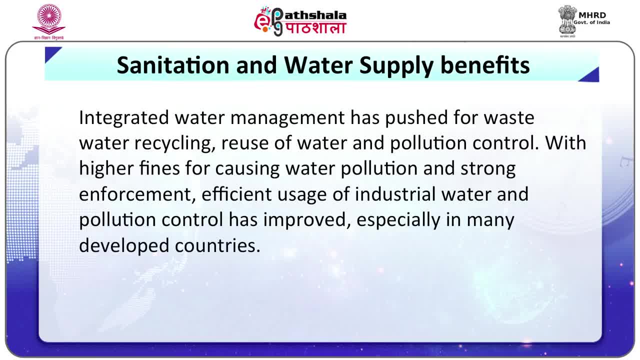 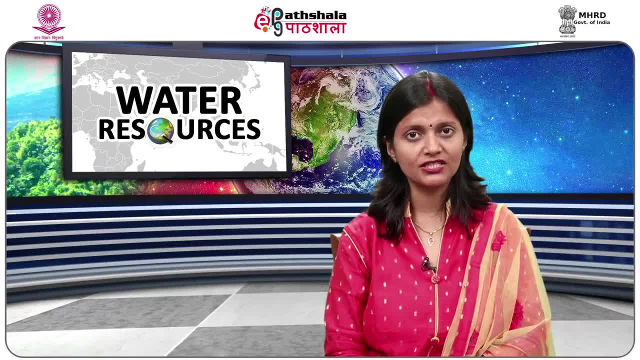 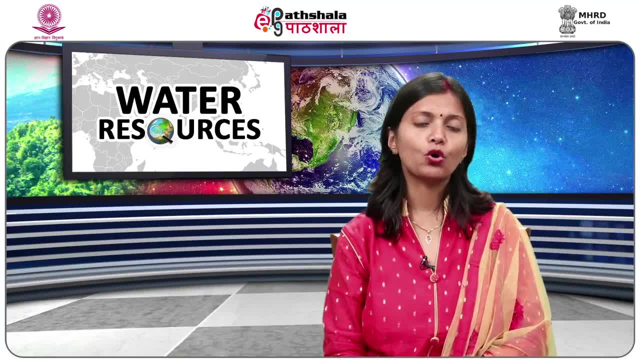 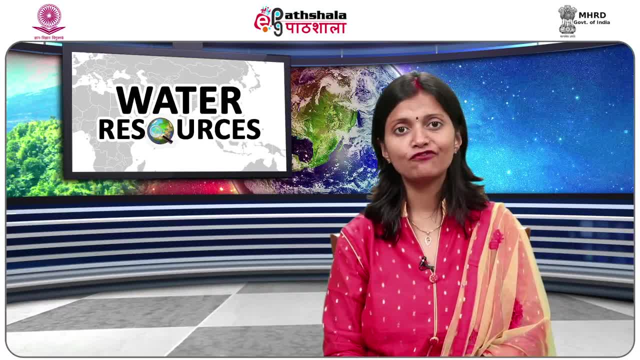 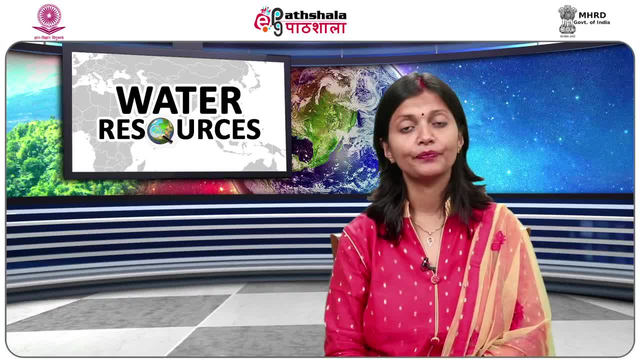 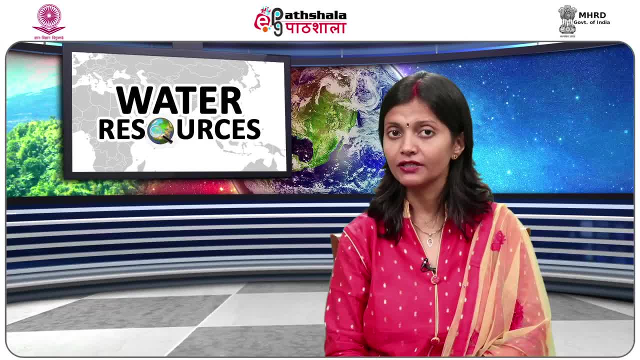 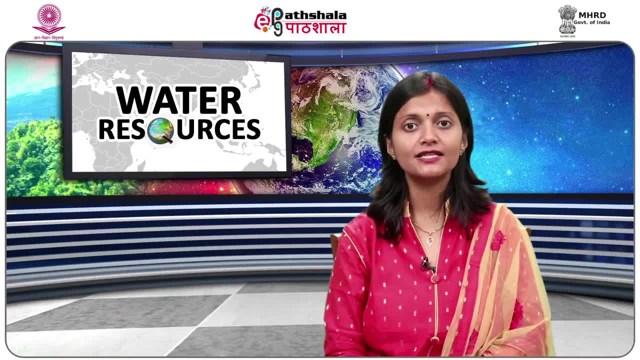 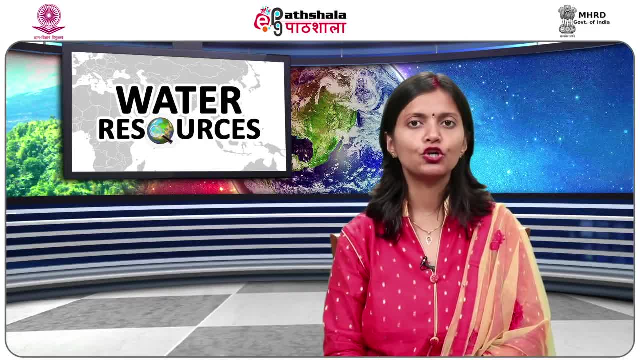 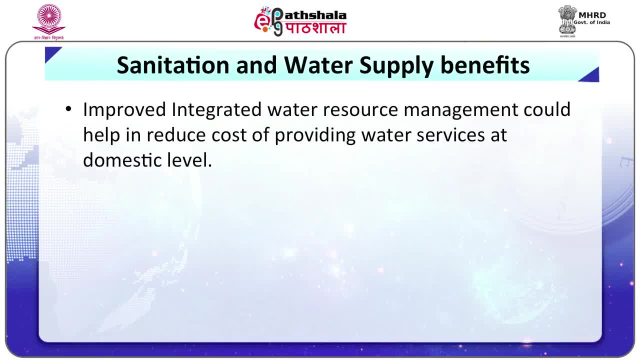 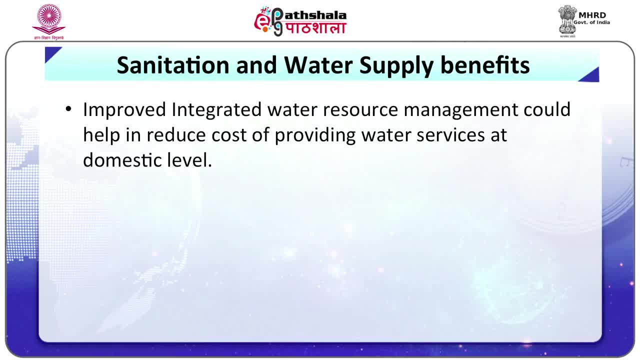 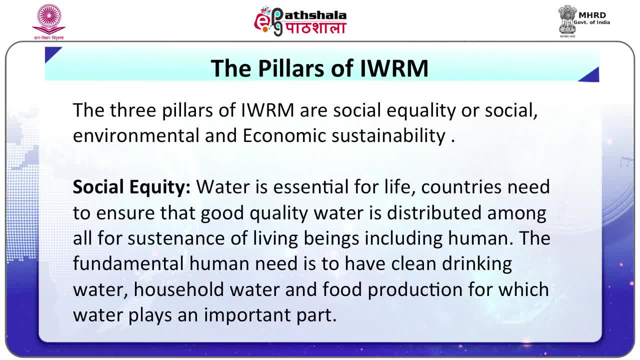 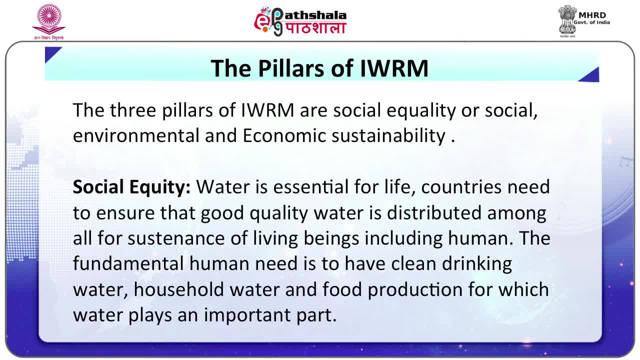 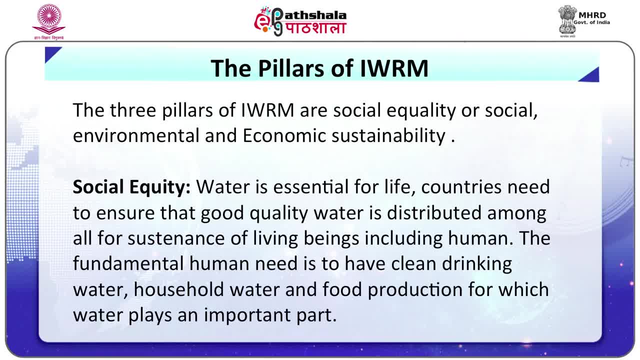 The approach of IWP is to ensure the sustainable development of water resources. The approach of IWP is to ensure the sustainable development of water resources. The approach of IWP is to ensure the sustainable development of water resources and economic sustainability. Social equality- Water is essential for life. Countries need to. 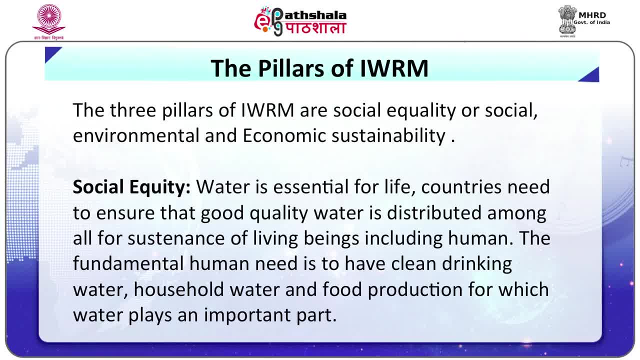 ensure that good quality water is distributed among all four sustenance of living beings, including human. The fundamental human need is to have clean drinking water, household water and food production, for which water plays an important part. However, due to current mismanagement of 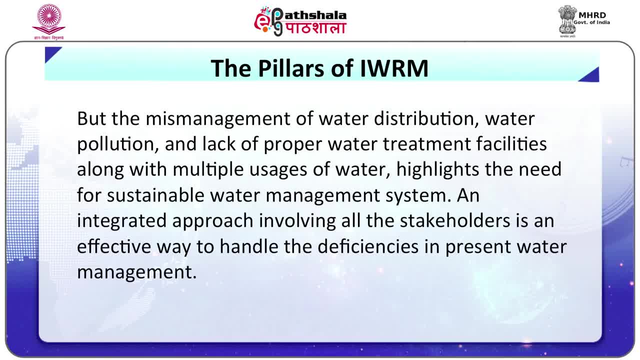 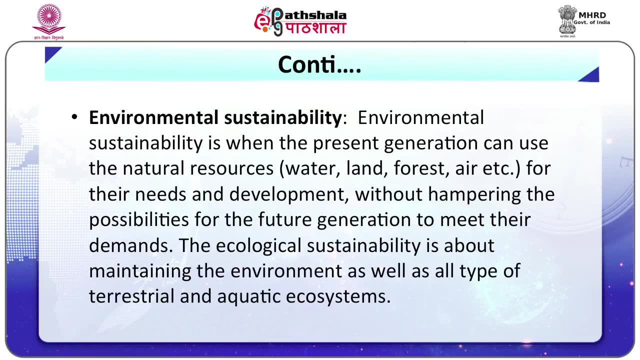 water distribution, water pollution, lack of proper water treatment facilities and also multiple usages of water, a sustainable water management system is required. An integrated approach involving all the stakeholders is an effective way to handle the deficiencies in present water management. Environmental sustainability is the another pillar of 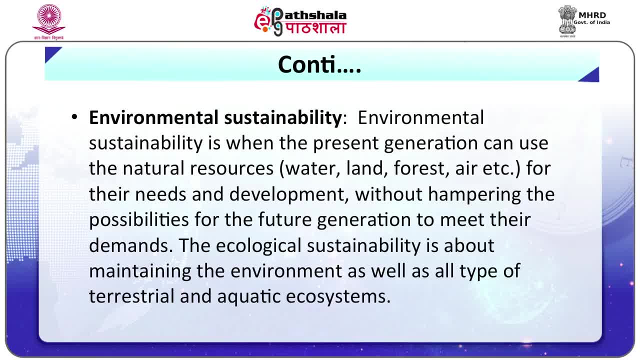 integrated water resource management. This is when the present generation can use. environmental sustainability is when the present generation can use the natural resources- water, land, forest, air, etc. for their needs and development without hampering the environmental sustainability of the present generation. 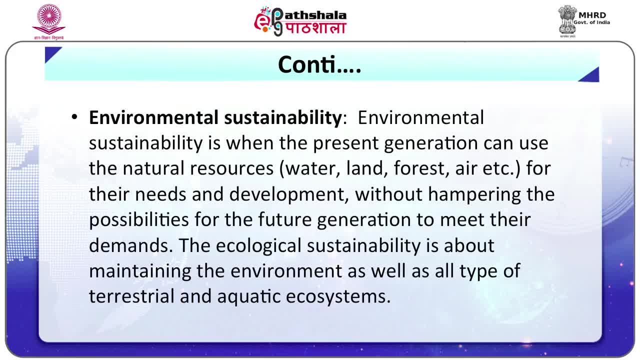 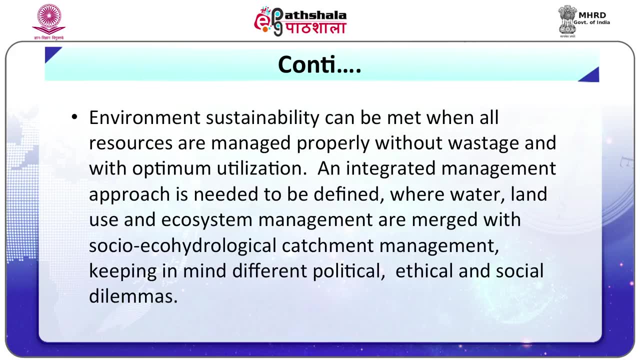 The ecological sustainability is about maintaining the environment as well as all types of terrestrial and aquatic ecosystems. Environment sustainability can be met when all resources are managed properly, without wastage and with optimum utilization. An integrated management approach is needed to be defined, where water, land use and ecosystem management are merged with socio-eco-hydrological. 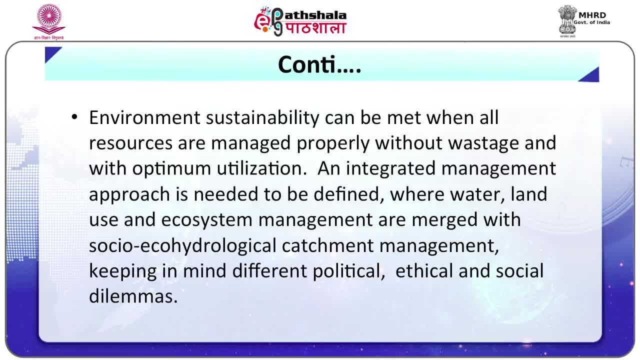 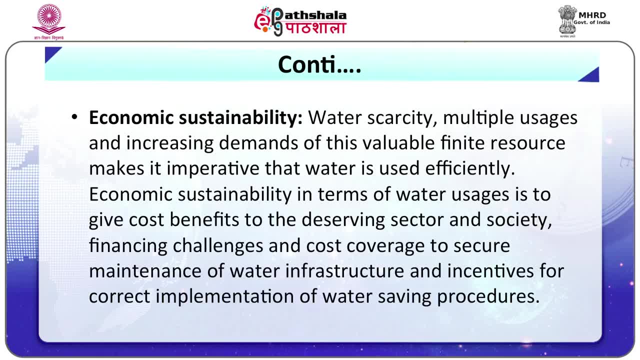 catchment management, Keeping in mind that all resources are managed properly without yesterday becoming too laborious. The third pillar is economic sustainability. Water scarcity, multiple usages and increasing demand of this valuable finite resource makes it imperative that water is used efficiently. 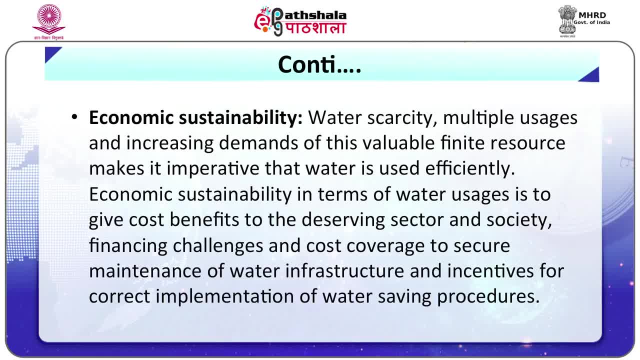 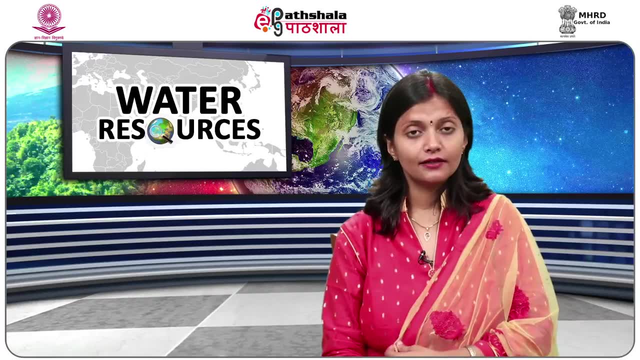 Economic sustainability in terms of water usage is to give cost benefits to the deserving sector and society. Financing challenges and costs are coverage to secure a maintenance of water infrastructure and incentives for customers. Dear audience, I welcome every for current implementation of water saving procedures. now let's understand. 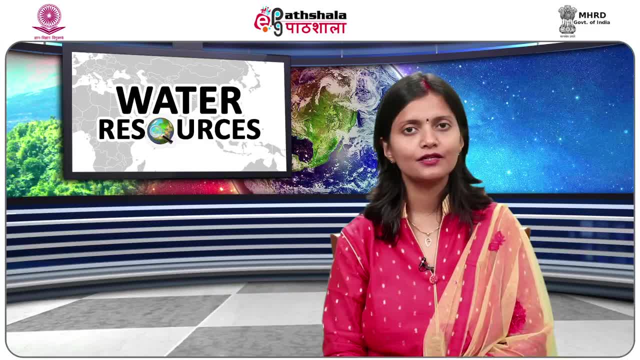 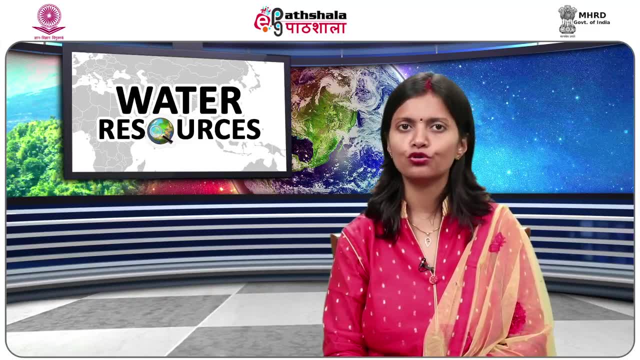 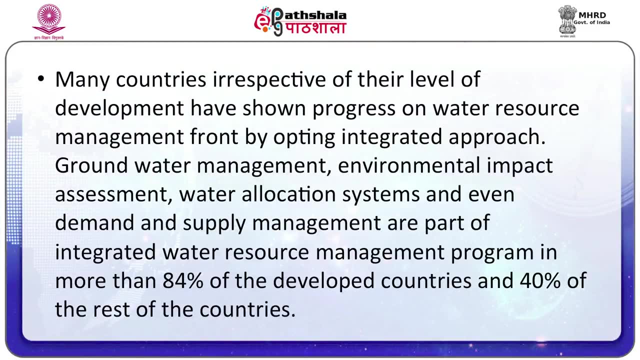 and discuss the status report of implementation of integrated water resource management approach across the world. the status report shared by UN water 2012 on integrated water management approach shows that about 60 percent of the world countries today have implemented strong water resource monitoring systems. many countries, irrespective of their level of 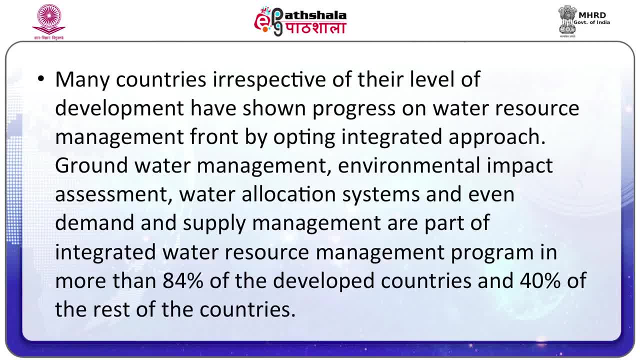 development have shown progress on water resource management front by opting integrated approaches. ground water management, implant environmental impact assessment, water allocation systems and even demand and supply management are part of integrated water resource management program in more than 84 percent of the developed countries and 40 percent of the rest of the countries. 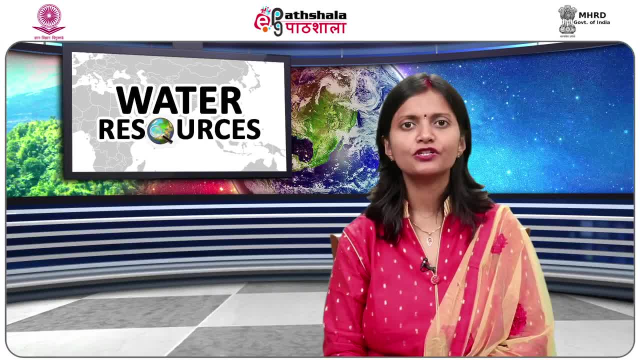 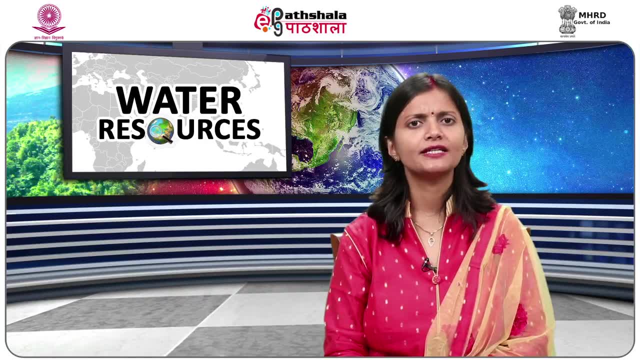 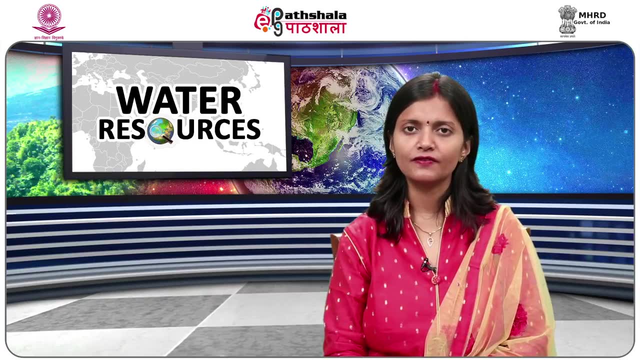 in terms of infrastructure development, more than 65 percent of the world countries have implemented advanced hydropower and water supply infrastructure, but only few have implemented advanced rainwater harvesting, irrigation and natural gas management and water management in the world. natural systems of water harvesting. the scope of improving infrastructure. 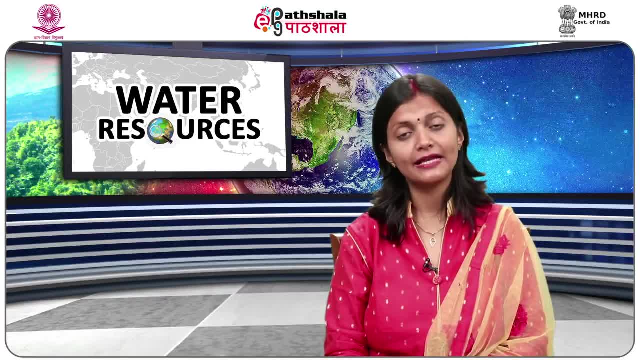 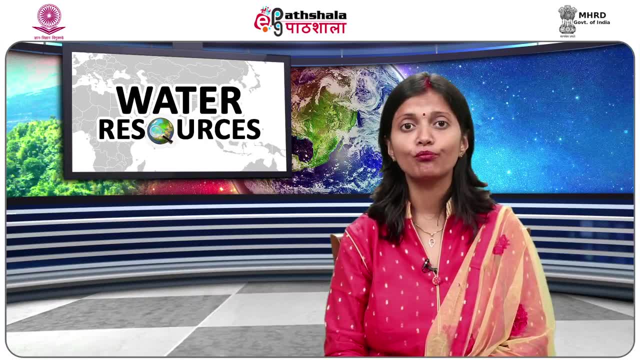 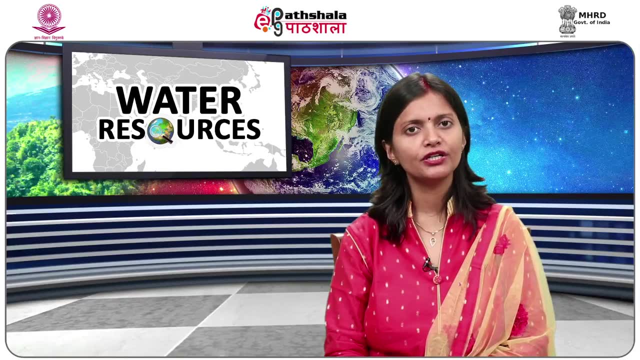 development, along with integrated approach, is still immense in many developed as well as developing countries. the financing survey for water resource development shows many countries have more moved forward in direction in financing for water resource development and management. about 50% of the lower income countries have shown increasing trend by their 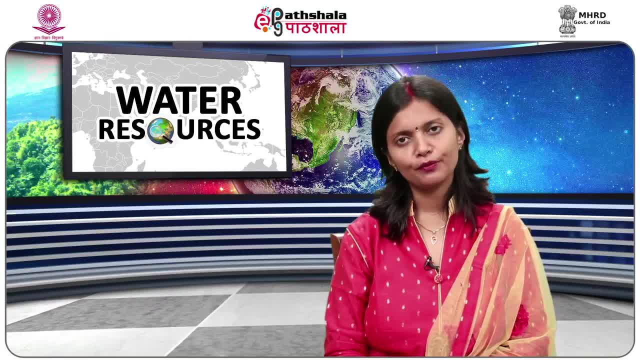 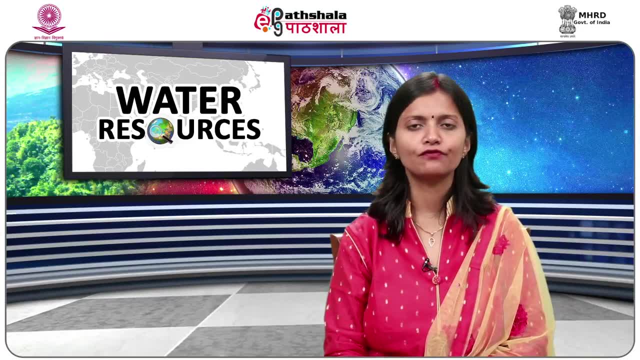 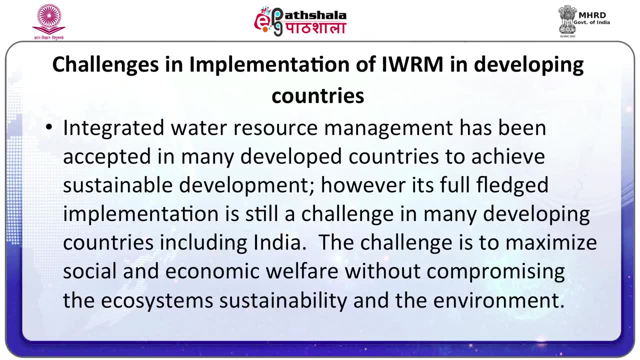 government to allocate more funds toward water development project- also funds from both users and polluters. however, much more needs to be done to improve the payment system for water management. now let's understand the challenges in implementation of IWRM in developing countries. integrated water resource management has been accepted in many developed countries to achieve 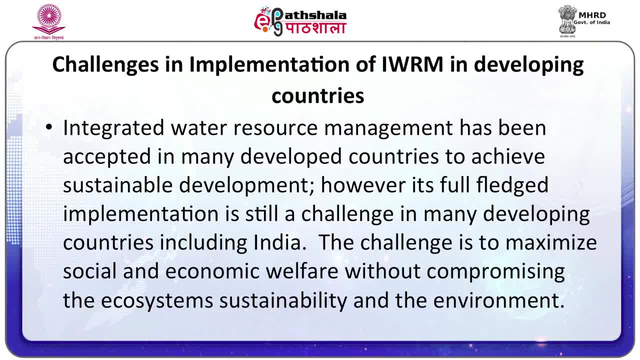 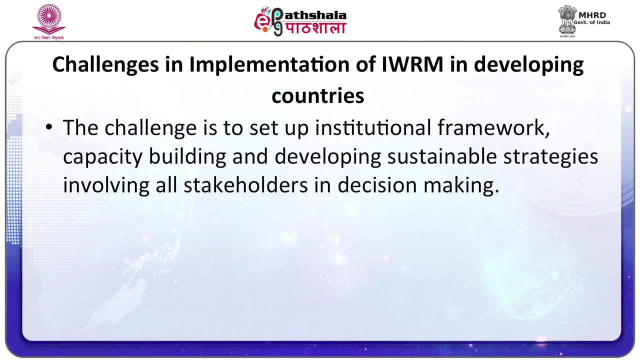 sustainable development. however, it's full-fledged implementation is still a challenge in many developing countries, including India. the challenge is to maximize social and economic welfare without compromising the quality of water and the environment. the challenge is to set up institutional framework, capacity building and developing sustainable strategies involving all stakeholders in 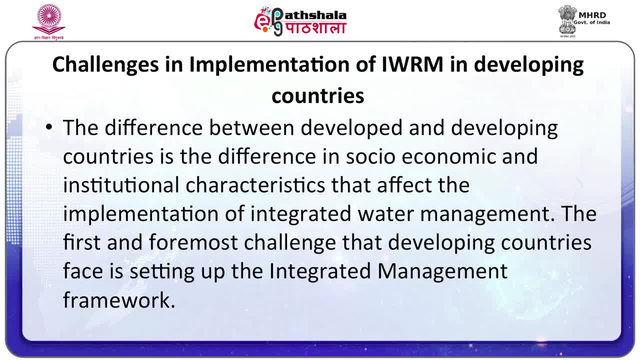 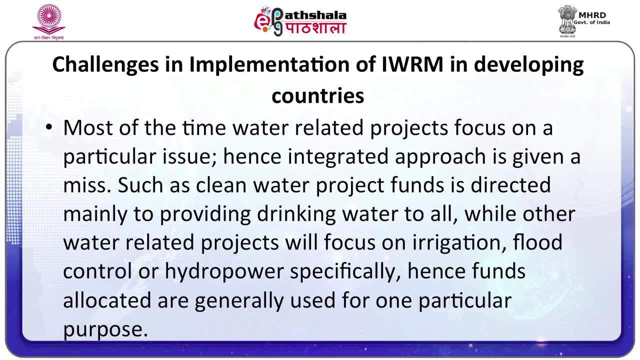 decision-making. the difference between developed and developing countries is the difference in socio-economic and institutional characteristics that affect the implementation of integrated water management. the first and foremost challenge that developing countries face is setting up the integrated management framework. most of the time, water related project focus on a particular issue, hence integrated approach is given a miss. such 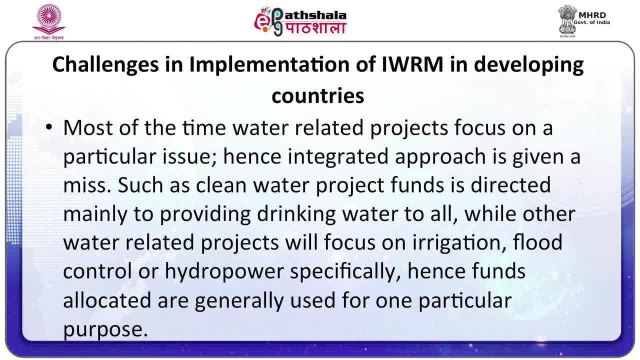 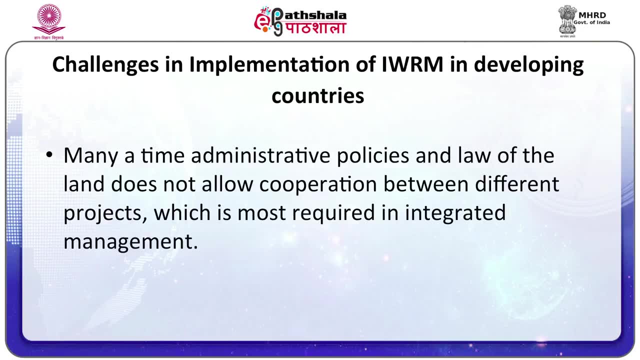 as clean water project fund is directed mainly to providing drinking water to all, while other water related projects will focus on irrigation, flood control or hydropower, specifically, specifically. hence funds allocated are generally used for one particular purpose many a time. administrative policies and law of the land does not allow cooperation between different projects, which is most 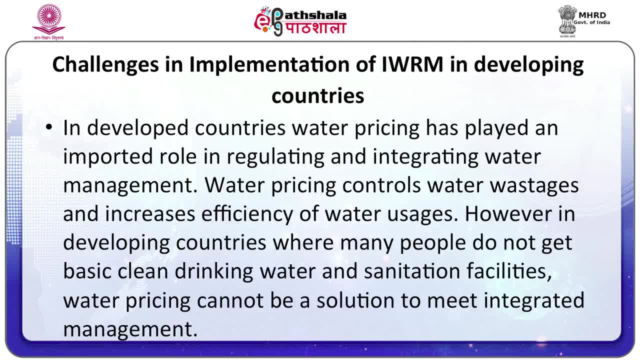 required in integrated management. in developed countries, water pricing has played an important role in regulating and integrating water management. water pricing controls water wastages and increases efficiency of water usages. however, in developing countries, where many people do not get basic clean drinking water and sanitation facilities, water pricing cannot be a solution to meet integrated management. 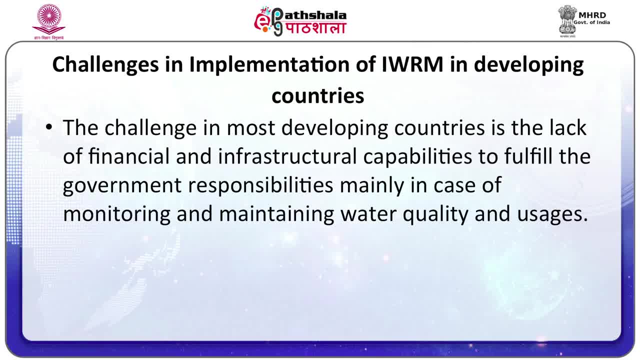 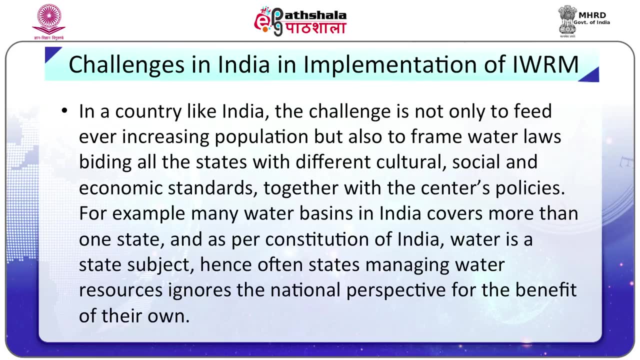 the challenge in most developing countries is the lack of financial and infrastructural capabilities to fulfill the government responsibilities, mainly in case of monitoring and maintaining water quality and usages. in a country like India, the challenge is not only to feed ever-increasing population, but also to frame water laws. 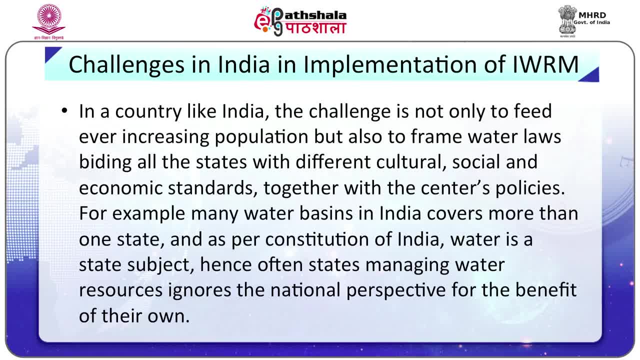 by adding all the states with different cultural, social and economic standards, together with these centers policies. for example, many water bases in India covers more than one state and, as per the Constitution of India, water is a state subject. hence, often states managing water resource ignores the national perspective for the benefit of their own. the integrated approach, though, may be, 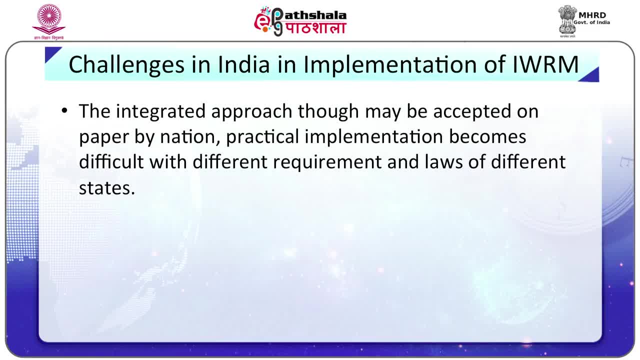 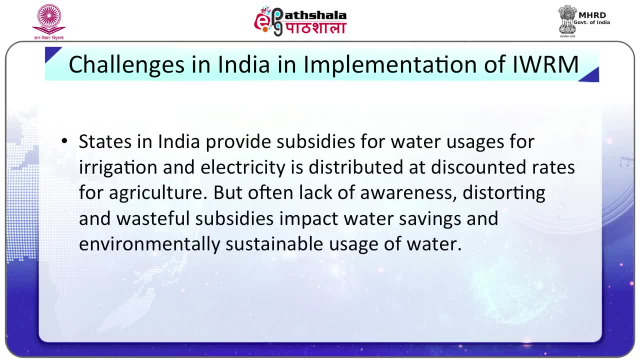 accepted on paper by nation. practical implementation becomes difficult with different requirement and laws of different states. states in India provide subsidies for water usages for irrigation and electricity is distributed at discounted rates for agriculture. but often lack of awareness, distorting and wasteful subsidies impact water savings and environmental sustainable usage of water. 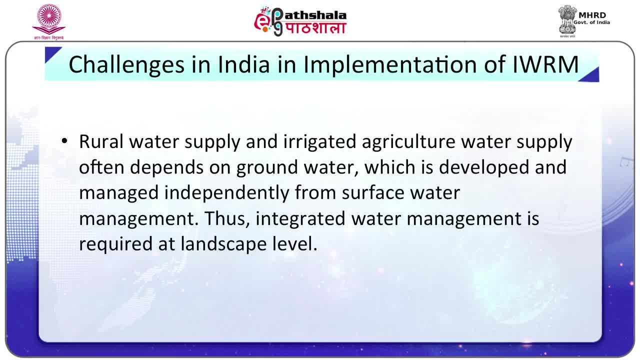 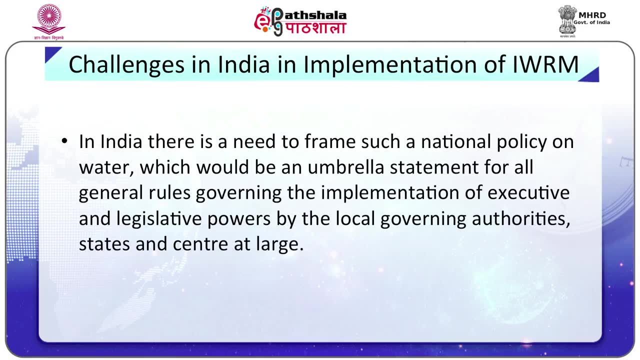 rural water supply and irrigated agricultural water supply, often different, depends on groundwater which is developed and managed by India and the rest of the world. India's water management is required at landscape level in India. there is a need to frame such a national policy on water, which would be an umbrella statement for 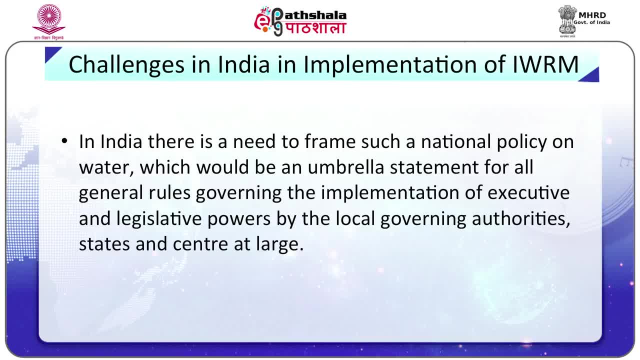 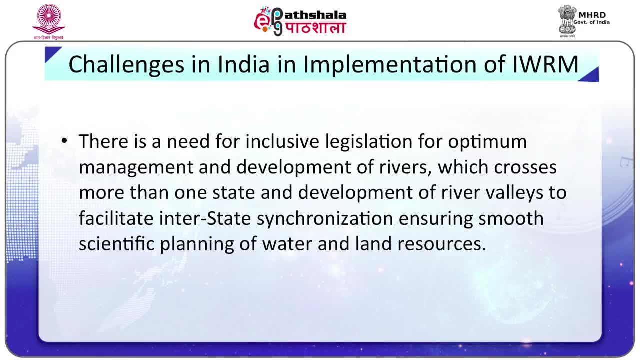 all general rules governing the implementation of executive and legislative powers by the local governing authorities, states and center. there is a need for inclusive legislation for optimal management and development of rivers which crosses more than one state and development of river valleys to facilitate interstate synchronization, ensuring smooth scientific planning of water. 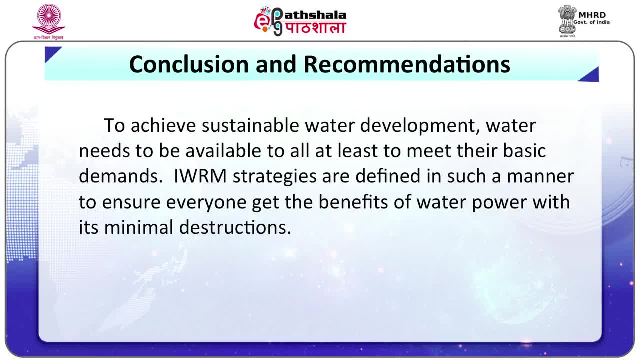 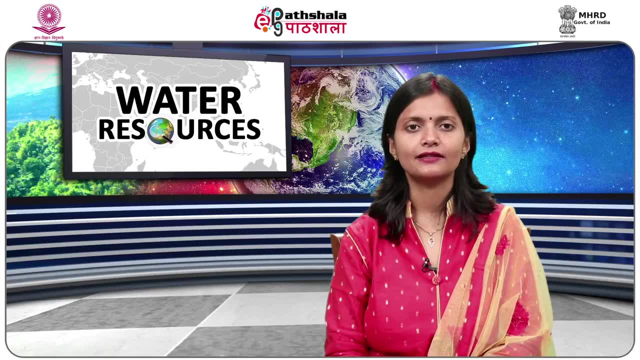 and land resources. Now to conclude, I can say, to achieve sustainable water development, water needs to be available to all, at least to meet their basic demands. Water secure world is a necessity, As defined by UN Water. water security is the capacity of population to safeguard sustainable. 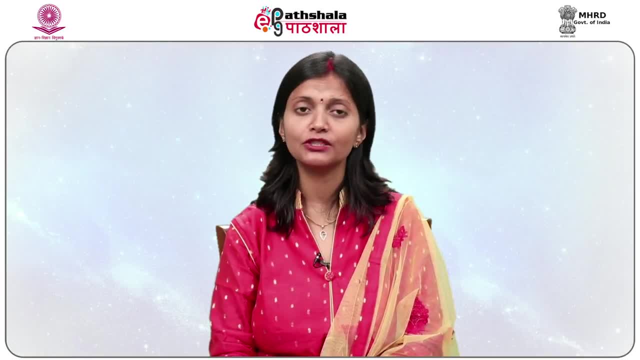 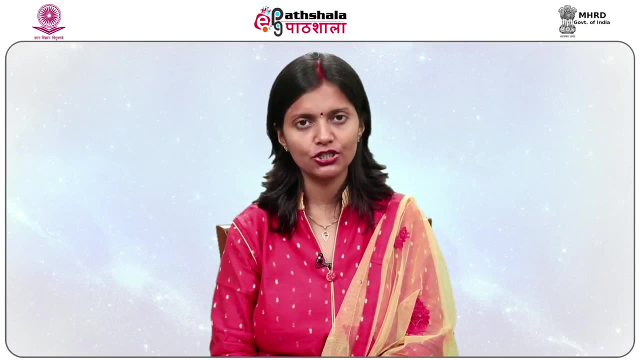 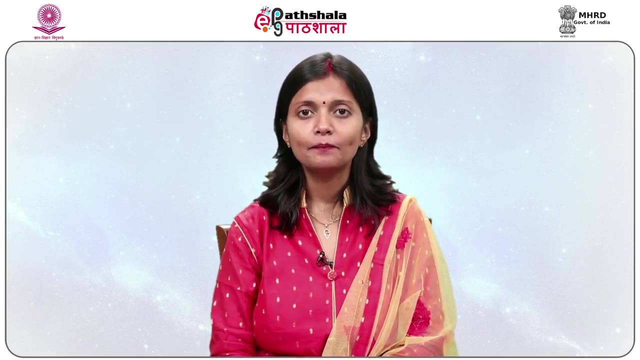 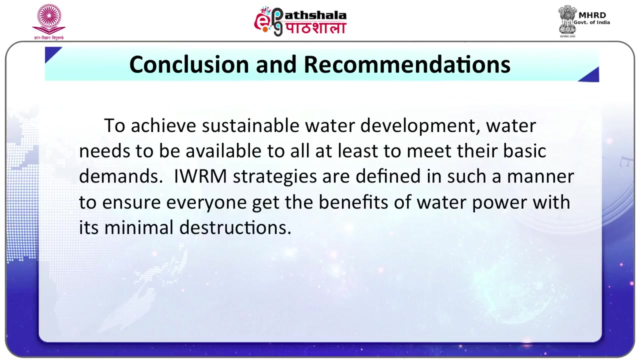 access to adequate quantities of acceptable quality water for sustaining livelihoods, human well-being and socio-economic development, for ensuring protection against waterborne pollution and water-related disasters, and for preserving ecosystems and a climate, peace and political stability. IWRM strategies are defined in such a manner to ensure everyone get the benefits of water. 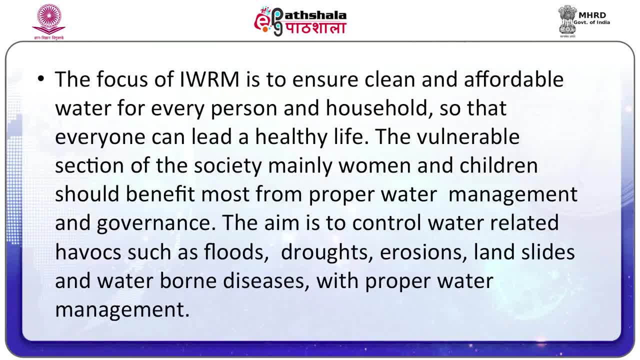 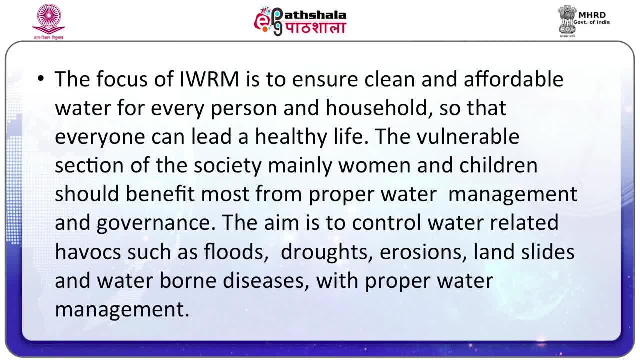 life. The vulnerable section of the society, mainly women and children, should benefit most from proper water management and governance. The aim is to control water-related havocs such as floods, droughts, erosion, landslides and waterborne diseases, with proper water management. 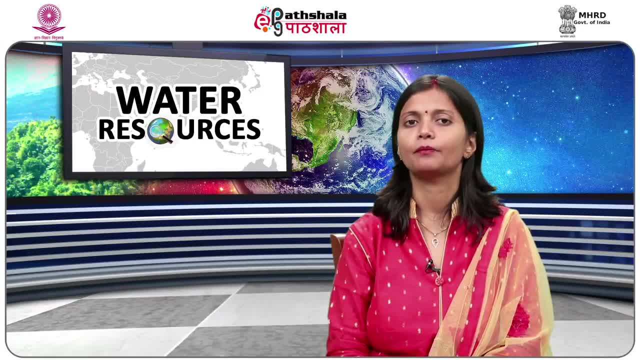 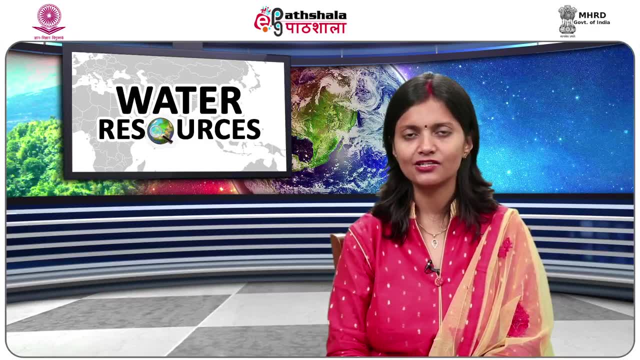 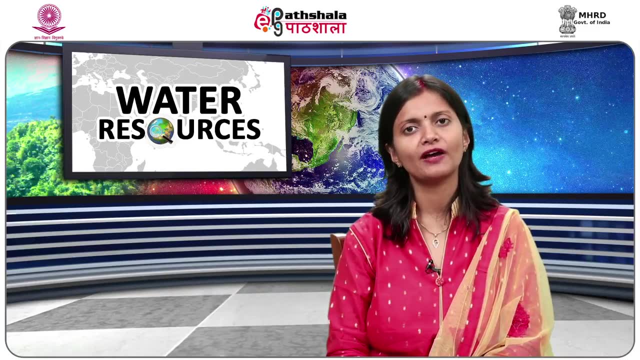 Water security in general would promote sustainable environmental development. IWRM brings all sectors of water management together, including agriculture, agriculture, energy industries, education, health, planning and finance. The joint effort of management by all sectors is the main focus of IWRM. Thank you, friends.